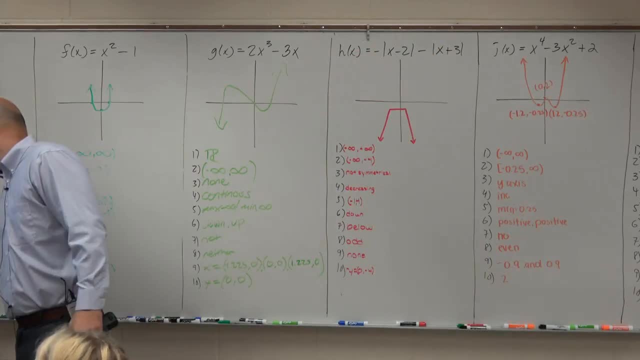 Okay. so in this example, ladies and gentlemen, you can see. here is what the graph looks like. You guys ready? Good, Okay, so there's on the graph. Now. the nice thing about Desmos is, obviously, we can go ahead and click on these points and you guys can see where the intercepts are, as well as. 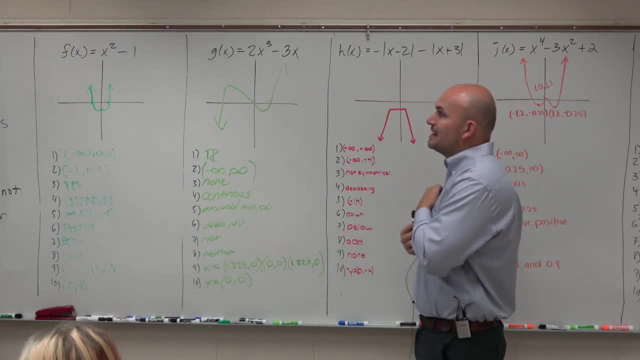 some max and some mins. All right, now let's kind of go through this step by step. On the first graph, the main thing- we guys- I'm going to have to move that desk If you guys need to move over here- 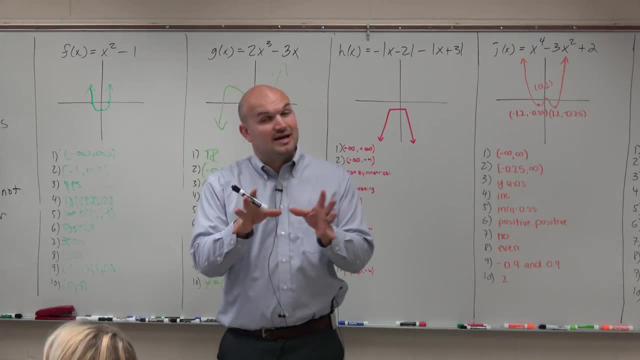 we can do that. So the first thing was you need to identify the domain and range Again. if you guys look at this, remember what we talked about last class period. just looking at the equation, There's nothing in. there's nothing that's going to make the denominator zero, or 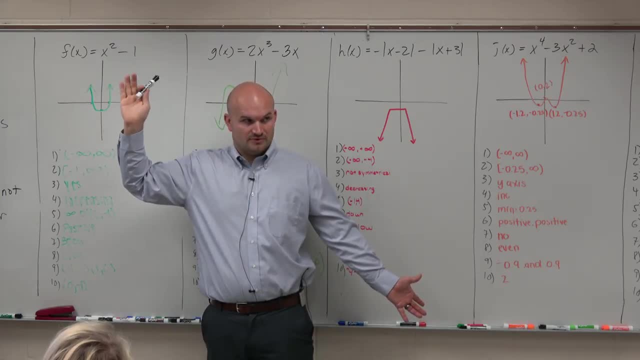 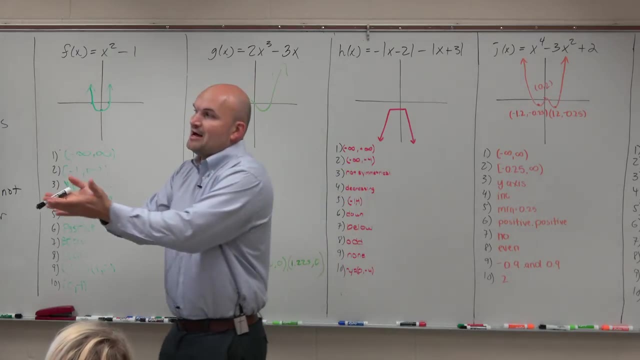 there's no radical there, right? So automatically- I'm really having trouble with this- So automatically we can see, we know that there's no values that are going to be discontinuous. And then obviously, looking at the graph, there's no reason for us to believe that the graph is not. 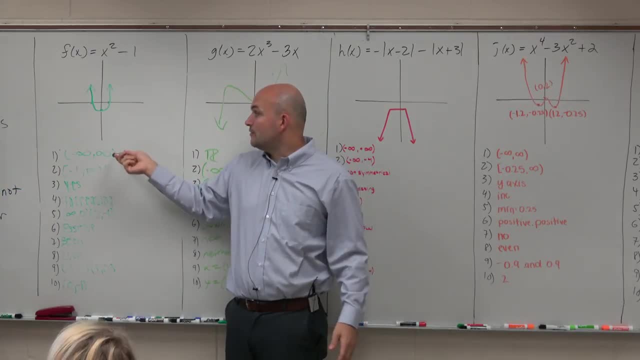 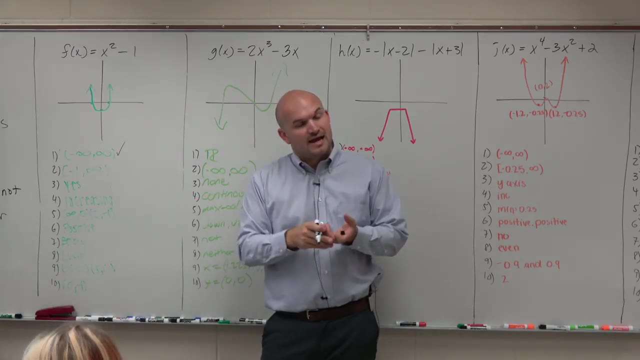 going to continue doing what it's doing: keep on expanding. So therefore, you can say that the domain is going to be from negative infinity to infinity. Good job, The range is going to be basically the set of all Y values And we're not going to talk about. 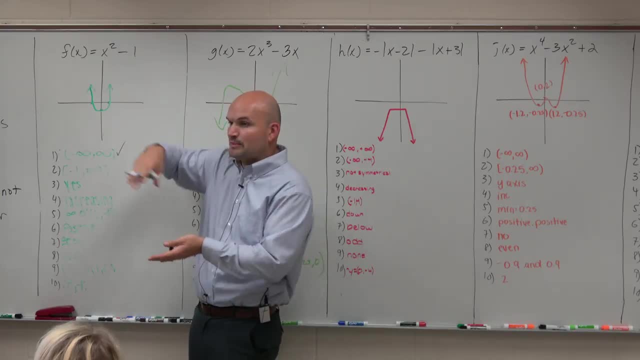 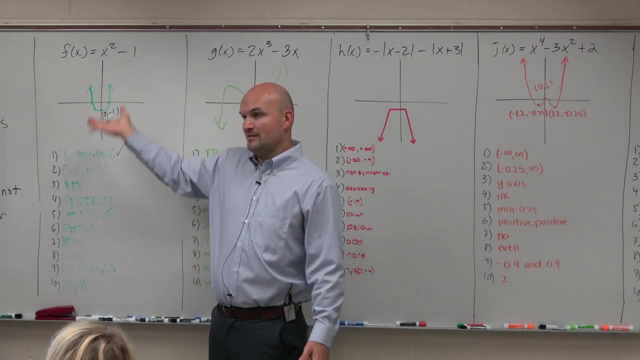 algebraically right now, but just geometrically. you can see from the graph: the lowest value the graph goes is at zero comma, negative one. So the lowest Y value is negative one, and then it's going to continue all the way up to infinity. So, range, good Symmetry, Yes. Well, I'm not really. 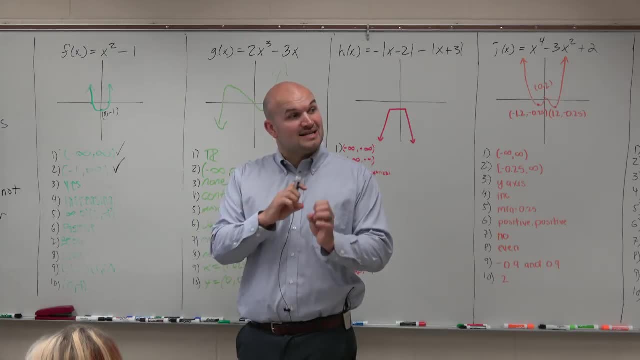 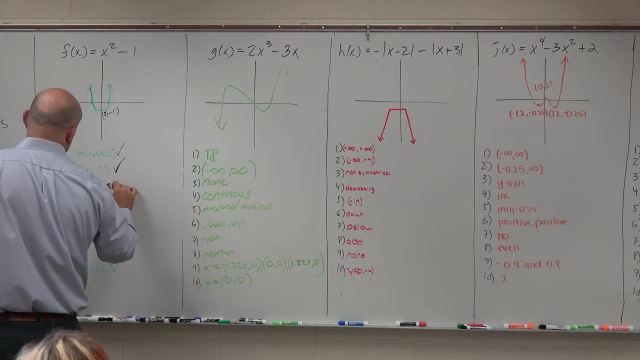 asking: is it symmetric? I'm saying: what is it symmetric about? So when you're asking the symmetry question, make sure you're telling me where is the symmetry. and it is symmetrical. I'll just write in about the Y axis. Okay, You guys can see there's that nice line of symmetry. 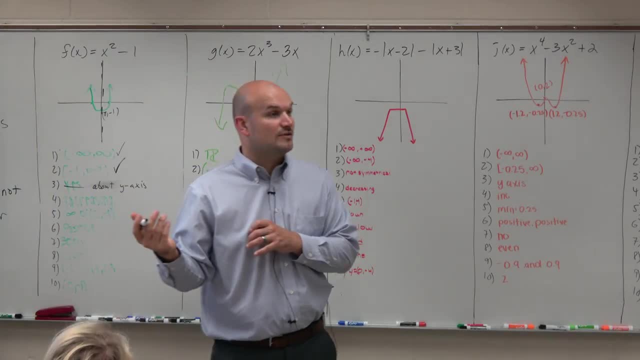 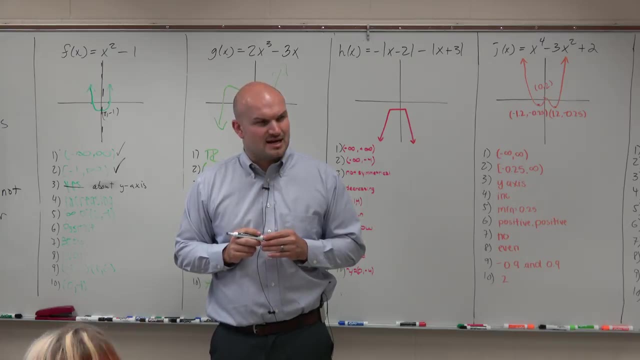 Whatever's on the left side of the Y axis, is this exact same on the right side of the Y axis? Okay, Again, we're having some other issues over there. The next one is increasing. I don't really understand if that means, because I actually I know that's not increasing. 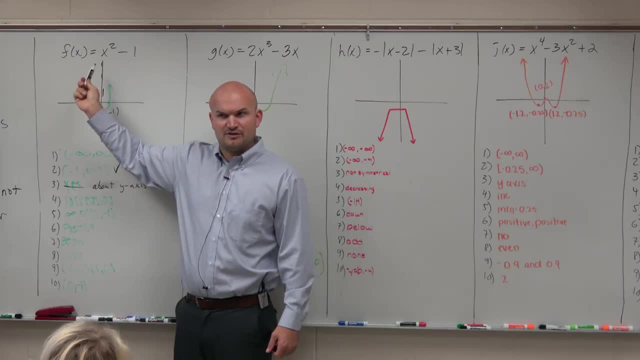 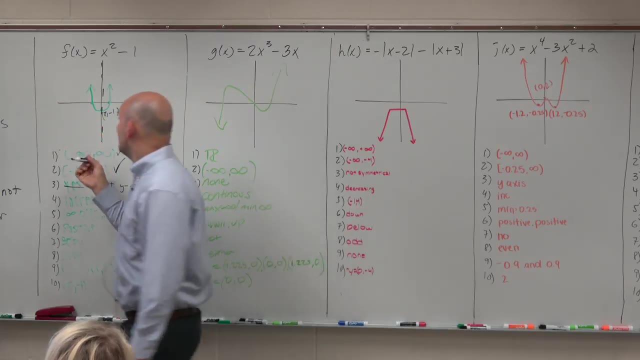 guys, As you read this graph to the left of the Y axis, is the graph increasing? Speaker 2: No, no, no. Speaker 1: As you're going from left to right, is the graph increasing? No, the graph is increasing. 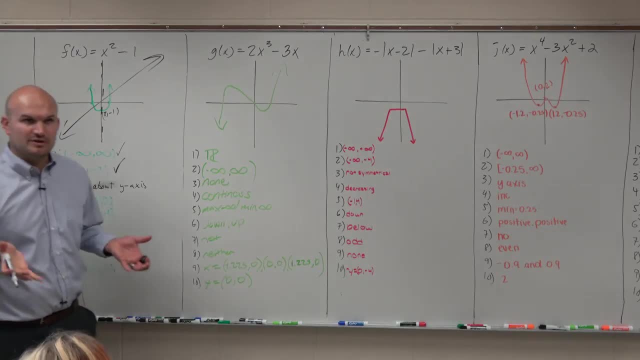 would look like this. That was a line, That was an algebra one, when the graph was increasing. This graph is not increasing. This graph is increasing from zero to infinity. So you could say it's increasing from zero to infinity. Now I will tell you guys, when we're doing interval notation for 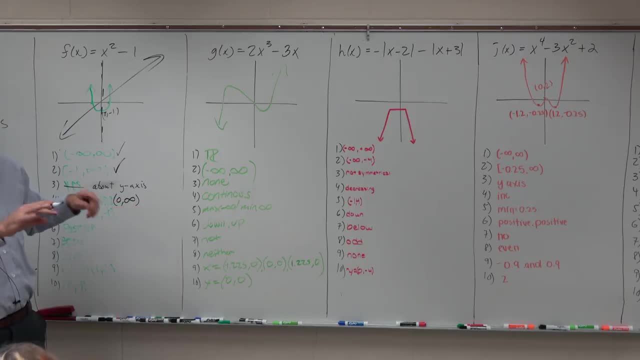 increasing, decreasing. you don't have to worry about the contains or the not contained. Remember how we did: like it's contained, not contained, You don't need to worry about that. for increasing, decreasing constant intervals: The graph is decreasing from negative infinity to 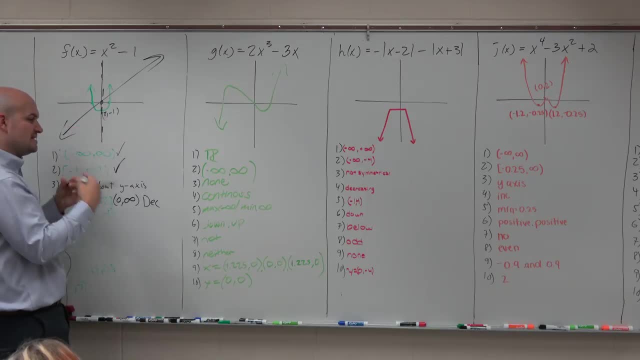 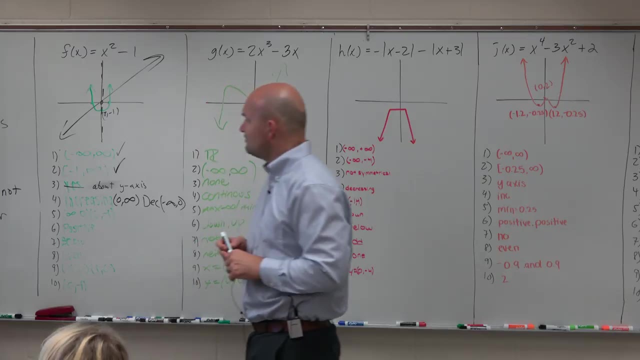 zero, The X value of zero. Again, we're talking about. what are the X values that the graph is increasing, decreasing, So that's going to be negative. infinity to zero. Number five is determine the max and the min points, So that's going to be points. We're trying to find an exact 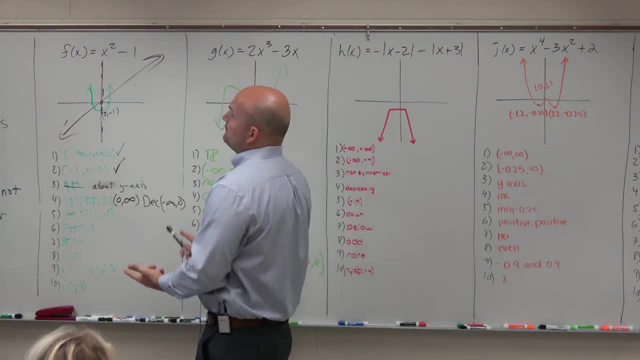 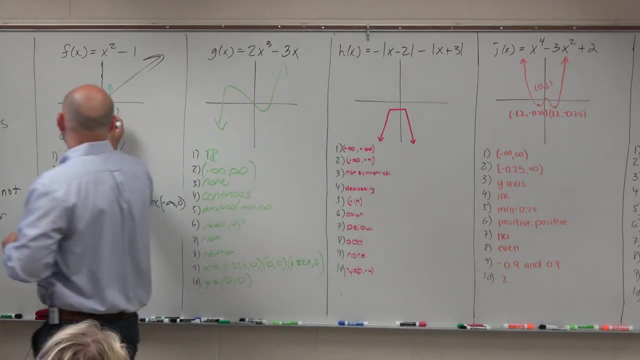 point where there is a maximum or a minimum value. Well, since the graph is shooting upwards, we know that the maximum there's going to be a minimum value. So we know that the maximum there's not going to be a maximum value. But as we're going down, you can see that from the left and 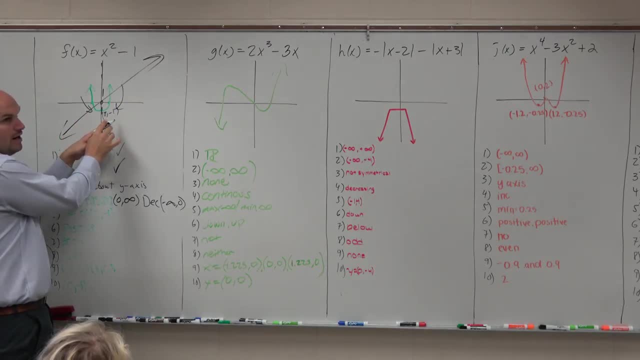 the right. the lowest point we get to is zero comma negative one. Now, that is the absolute lowest point this graph gets to correct. So therefore, this is actually what we call the absolute. I'm just going to use ABS- absolute minimum point, And that is going to be at zero. 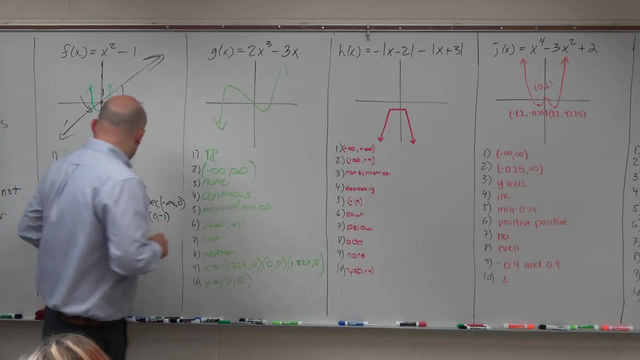 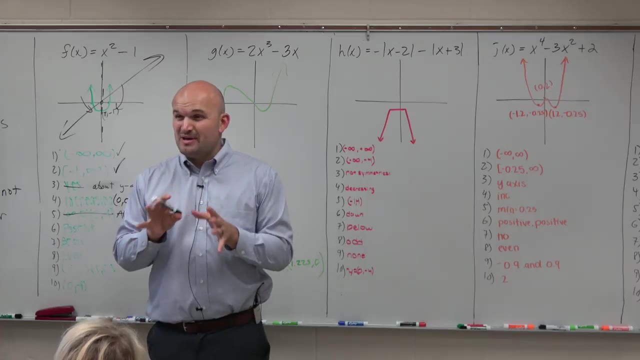 comma, negative one. Okay, Number six is going to be end behavior. So, guys, we're going to do end behavior, next chapter, in a little bit more detail, and you're probably not going to like the notation we're going to use, So I'm just going to revert. 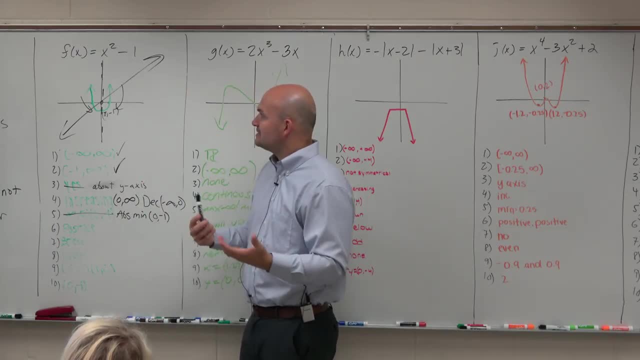 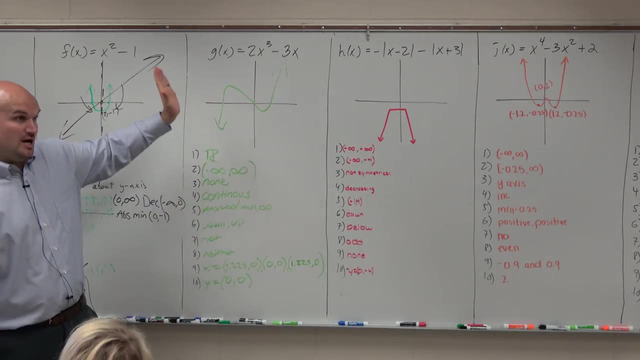 back to least algebra two stuff, Positive end behavior. I wouldn't really say that's the best. When you're describing end behavior, you want to say, as the graph, as the graph goes to the right, what is the graph doing? Is it going up or is it going down? The graph is going up, right. So 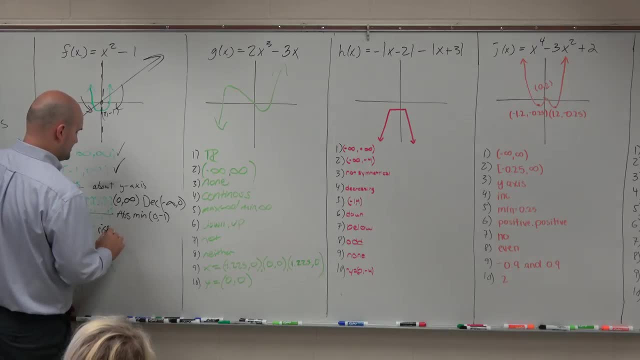 usually what we'd like to say is: you know, at least in algebra, two terms: it rises, you know, and rises left. Okay, But you want to give at least two different distinction. As the graph goes to the right, it goes up. As the graph goes to the left, it goes up. You want to at least make 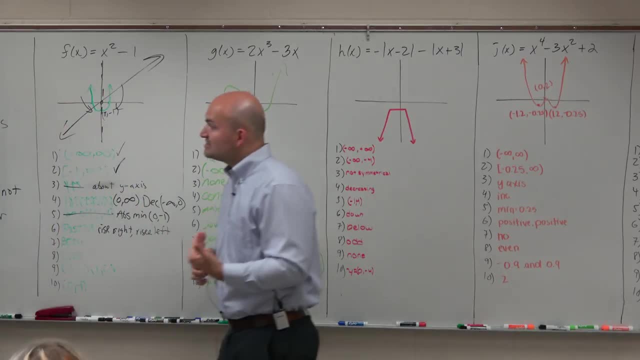 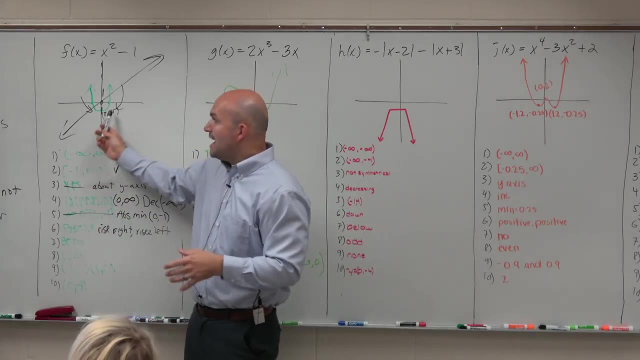 sure you're describing that when you're talking about end behavior- Number seven- we're talking about bounded. So again, think of bounded boundaries, right? Where is this boundary of this graph? Well, the graph, obviously, is unbounded going up, correct? But there's a boundary, is how? 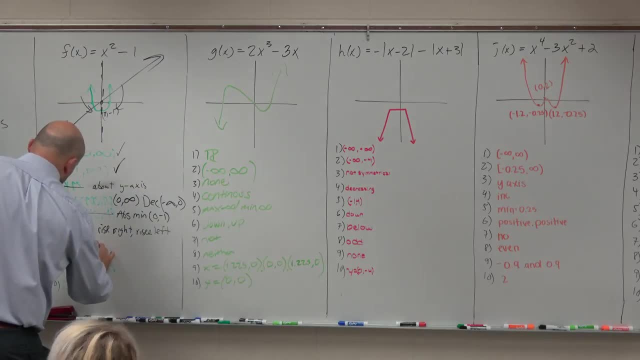 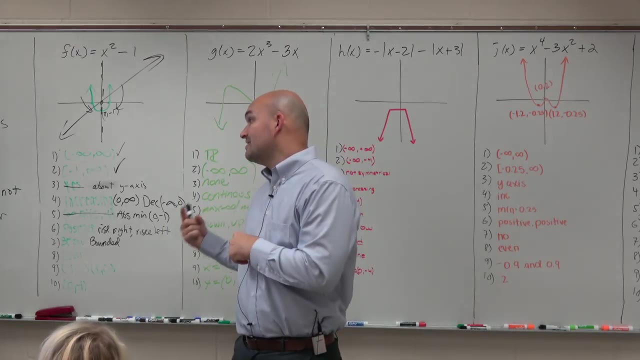 low it can go. So this is bounded below. So the head below, just make sure it's bounded below. The next one: is the graph even odd or neither? Well, guys, if you looked up the definition whenever the graph is reflexive. 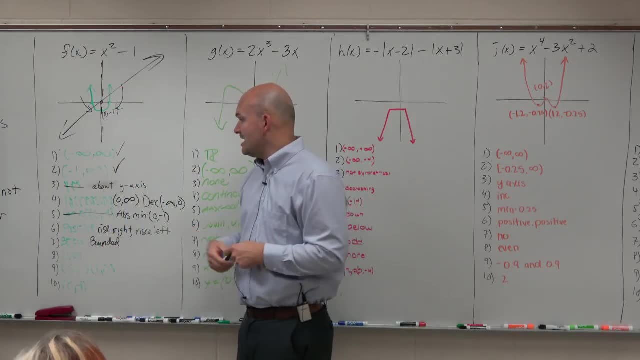 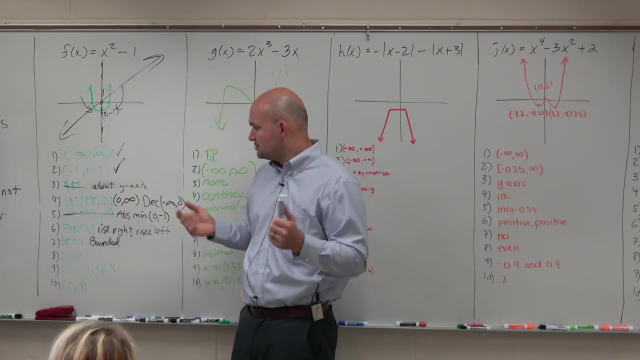 about the y-axis. it is even- Since this graph is reflexive- about the y-axis. it is even The x-intercepts. I just asked you to give the points or the values, but they gave me the points, which is perfectly fine. The x-intercepts are at negative one and one zero, and then the y-intercept. 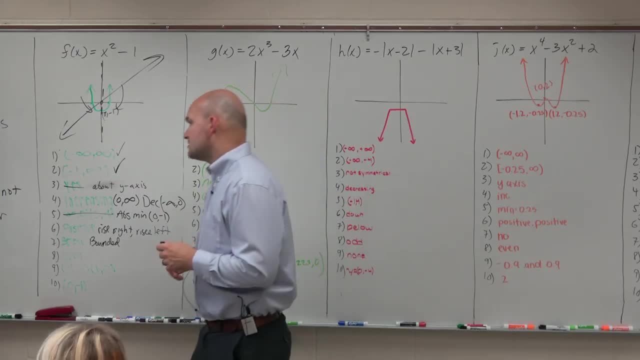 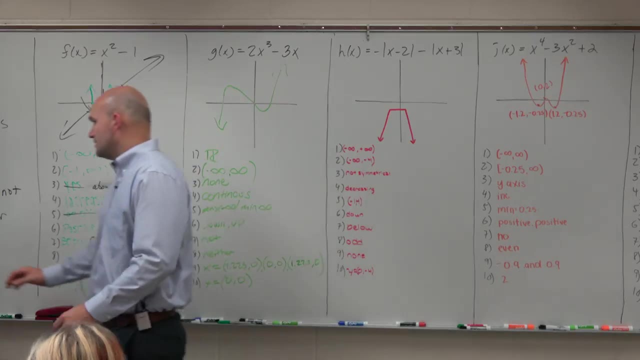 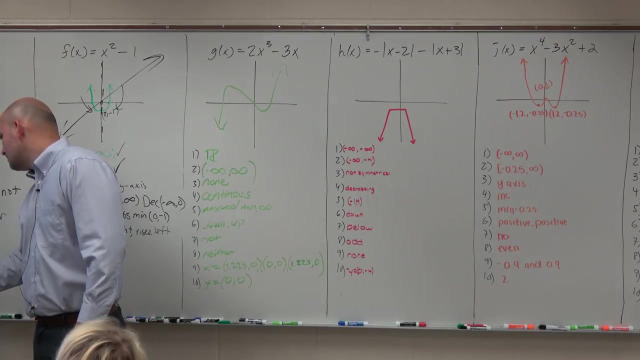 is zero comma negative one. That's perfectly fine. Okay, All right, So let's move on to the next one. So the next one is: Oh, I need to change that, don't I? This one? What'd you say? this is that one X minus one? All right, So in this graph Now. 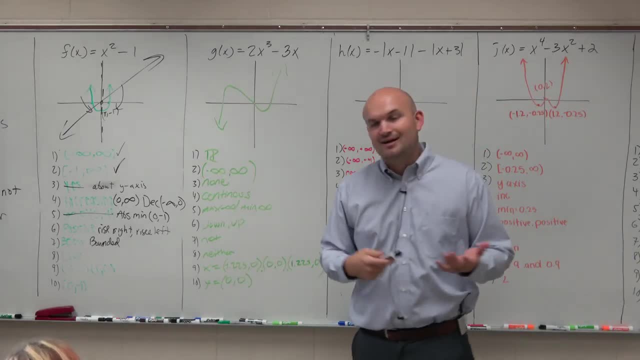 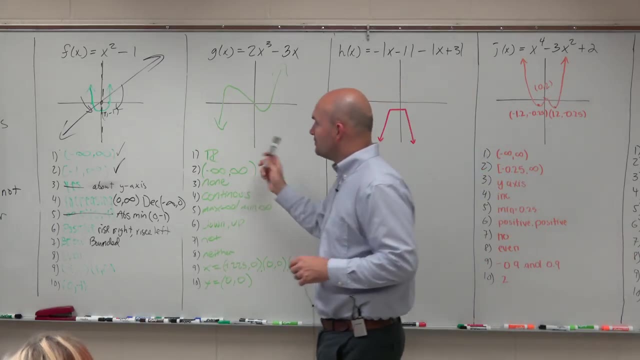 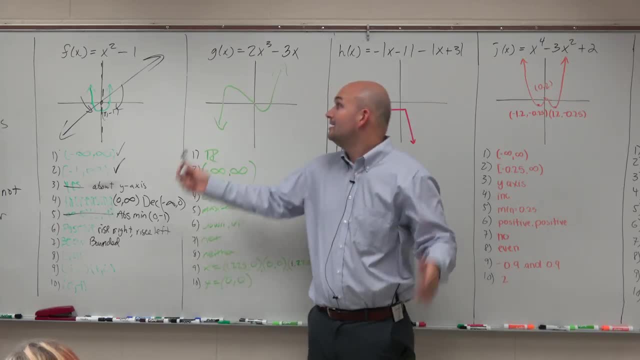 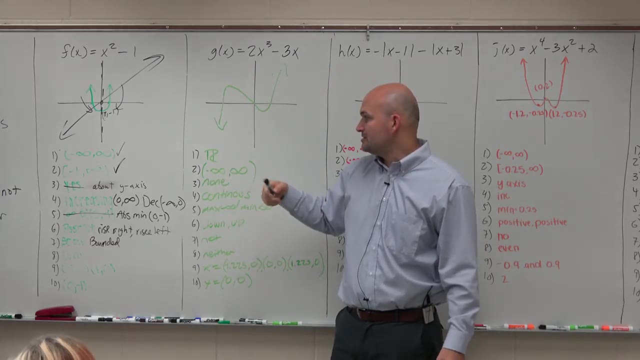 the domain, guys, you can see this graph is extending indefinitely. And the same thing algebraically. there's no denominator or radical that we need to worry about. So yes, the graph, the domain, is all real numbers. Then the range: you can see this graph is continuously going. 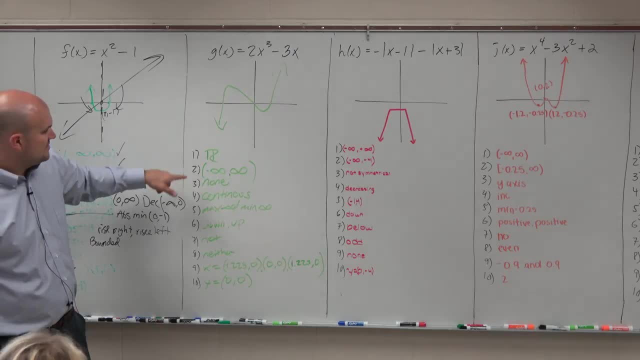 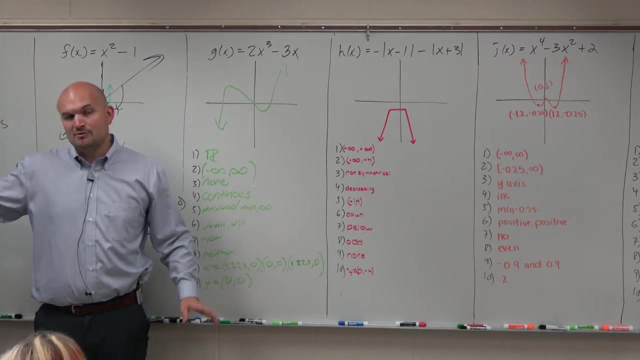 negative and positive, So that's also going to be all real numbers. For number three, we're looking at the symmetry. Now. this one's confusing. if you look at their graph, If you look at this graph, you might be able to visualize this better. It's not symmetric about. 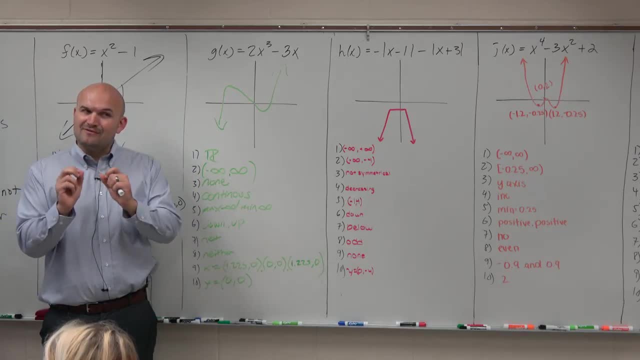 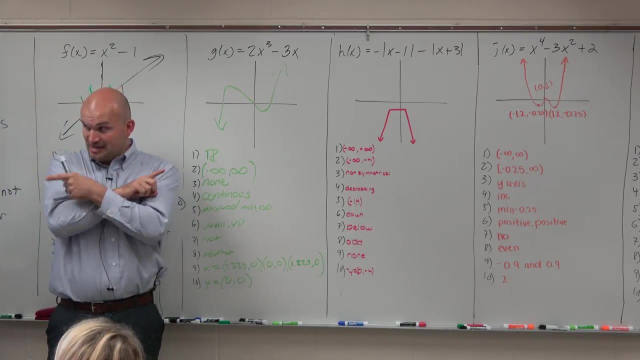 the x-axis, It's not symmetric about the y-axis. However, if you flip that graph about the x-axis and then flip it about the y-axis, could you guys see from that graph- I wouldn't really bet on that one- Do you guys see on that graph you're going to have exactly the same? Yes, So it's actually. 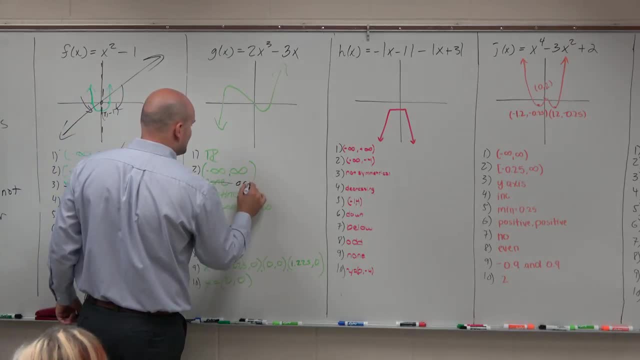 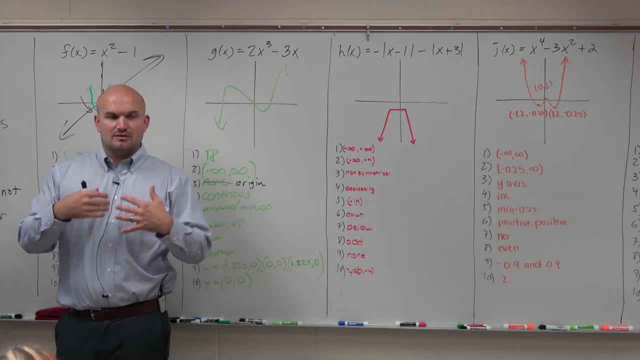 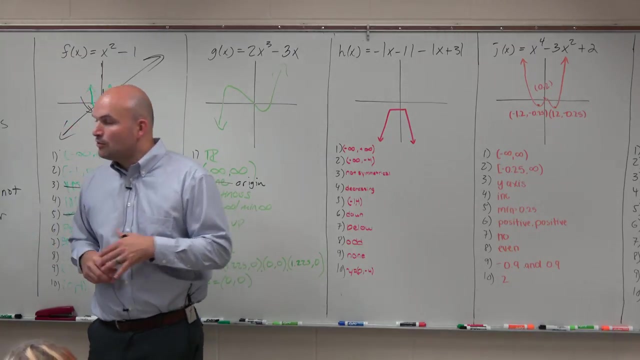 symmetric about the origin. So when we're talking about symmetry, just make sure you're not just saying, oh yeah, it's symmetric, What is it symmetric about? The next one is number four, which we're saying: is the graph increasing, decreasing or constant? 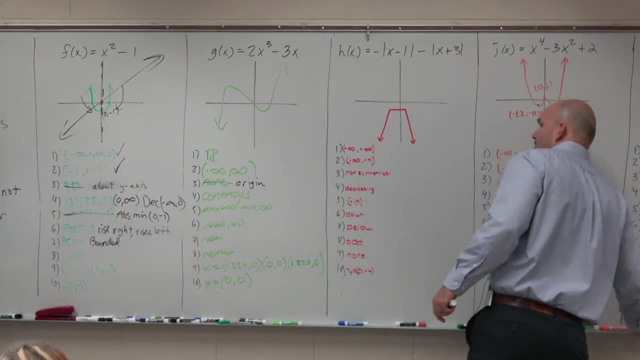 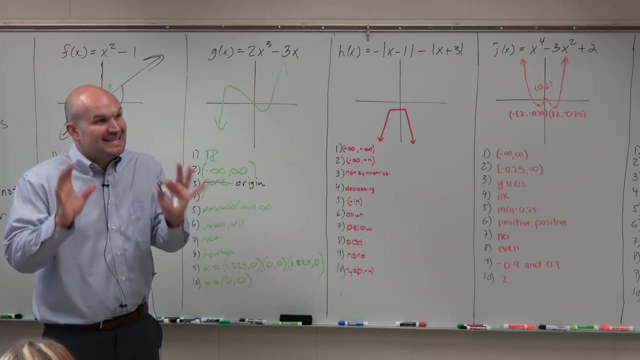 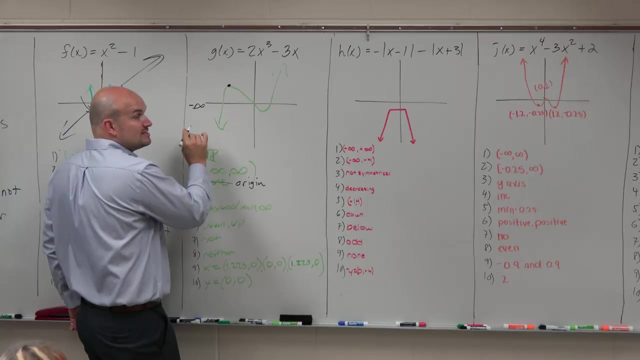 I'm not asking if it was continuous, That was constant. So again we're looking at the x values, The x values that the graph is increasing, decreasing, So all the way out here we're looking at negative infinity. This little turning point is at what Negative 1.2.. 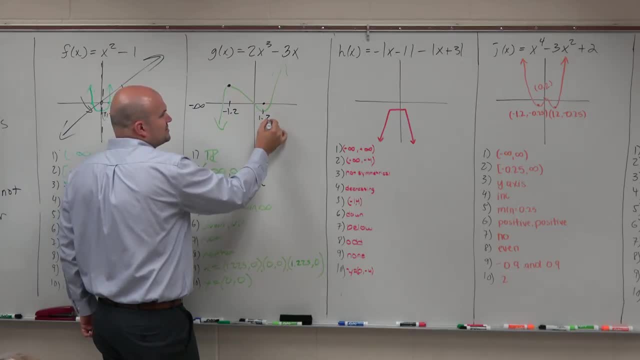 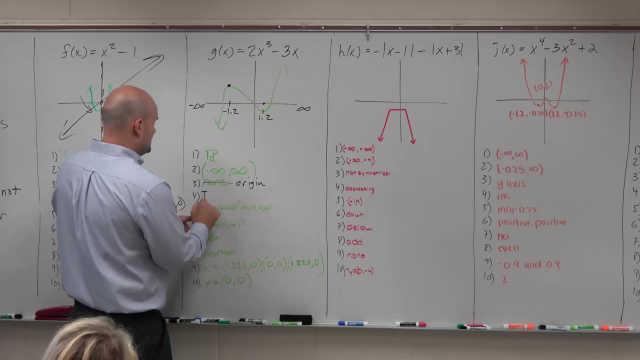 Then over here there's a number, Another turning point, which is at positive 1.2.. So you can see their graph is a little off, but that's OK. And then it goes to infinity. So the graph is increasing. On what values is? 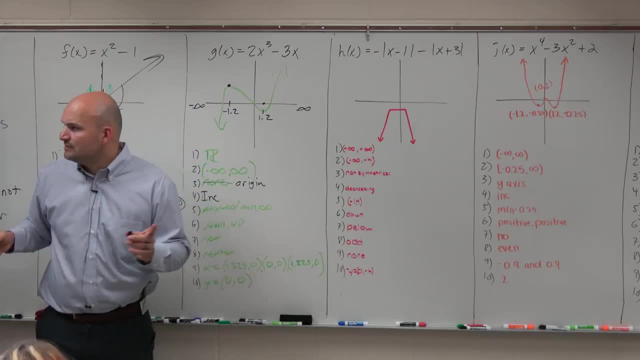 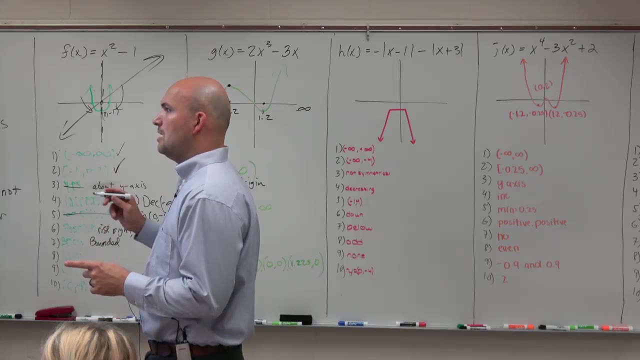 this graph increasing. Yes, It's 0.7.. Oh wait, negative 1.5.. Wait, what You were looking at, the x? Oh, thank you, I was looking at the wrong points. Negative: 0.7 and 0.7.. 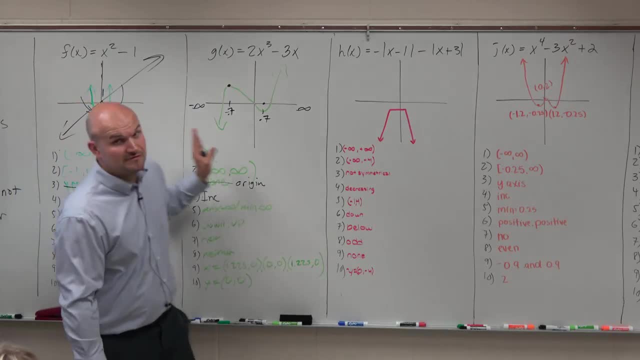 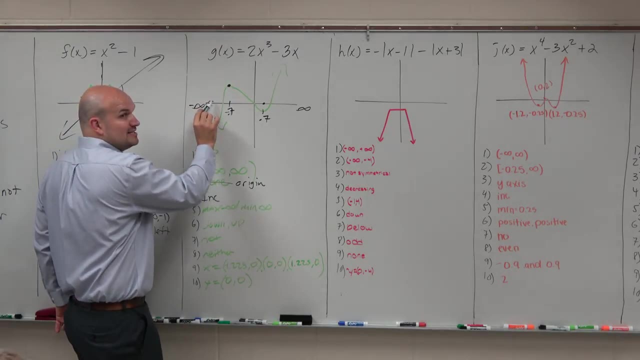 OK, So the graph is increasing. Remember, guys, we're reading the graph from left to right. This graph is increasing from the x values of negative infinity all the way to the x value of negative 0.7.. So you'd say negative infinity to negative 0.7.. And then it's also increasing. 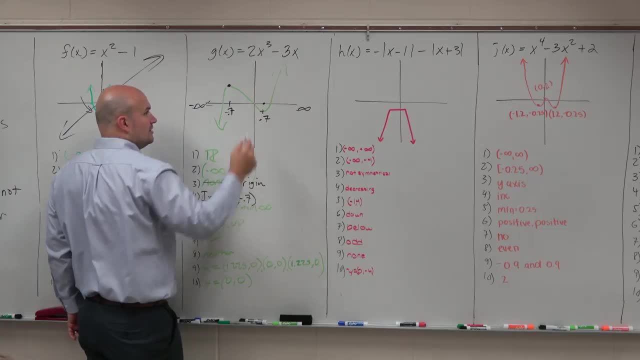 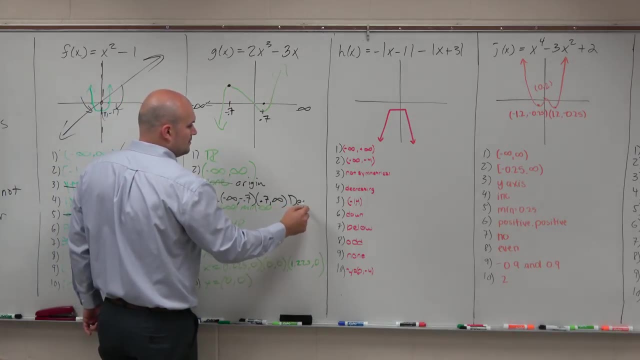 from this turning point, 0.7, to infinity, 0.7 to infinity. The graph is decreasing Between negative 0.7 and 0.7.. Do you guys see, You guys agree with me Between the x values. 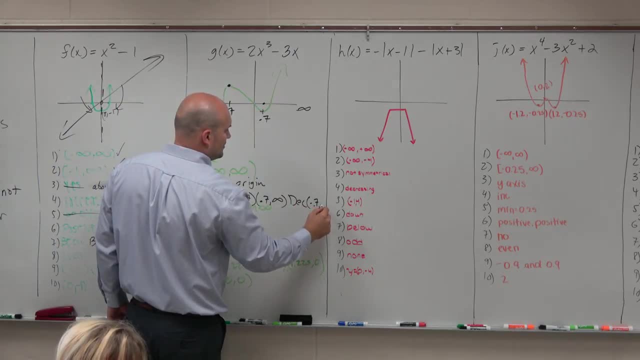 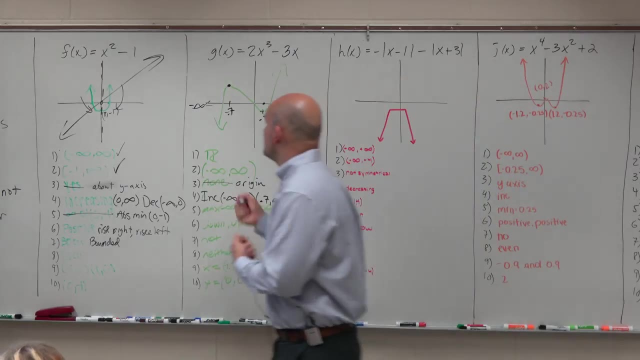 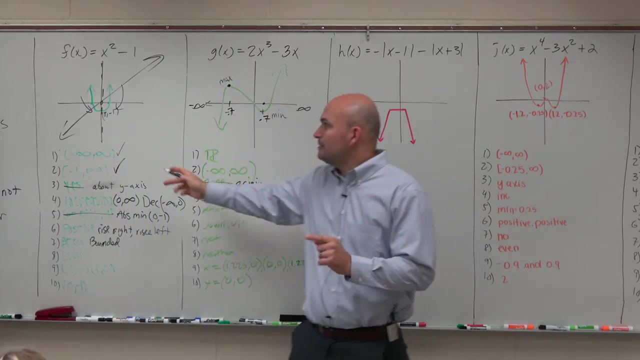 it's decreasing Negative 0.7 to 0.7.. All right, The next one was determine the max and the min points. So it looks like we have a maximum And it looks like we have a minimum. However, it's a little different than the last one. If you guys remember the last one, this was a minimum. 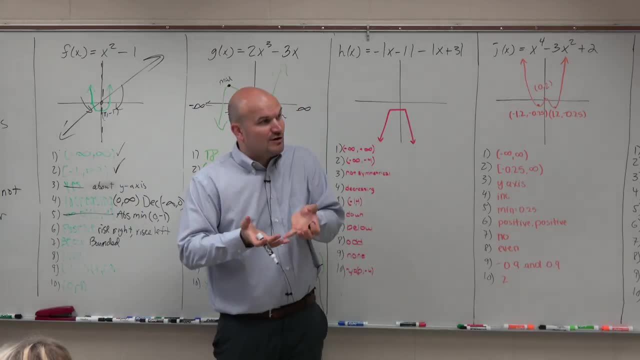 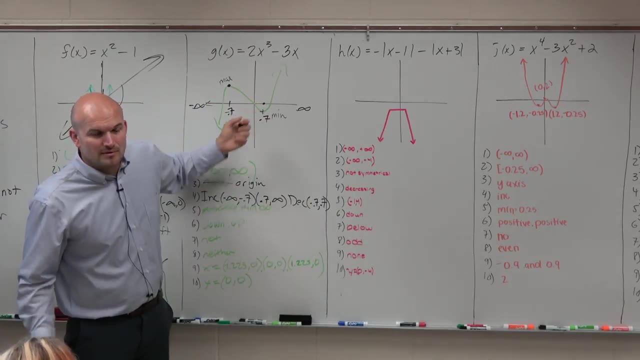 And we said this was the absolute minimum, because this was the absolute lowest that the graph went Correct. But when we look at this minimum, is this the absolute lowest that the graph is No Right. But here's kind of a cool thing. 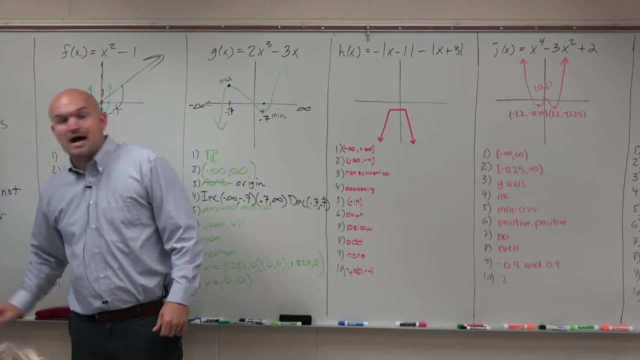 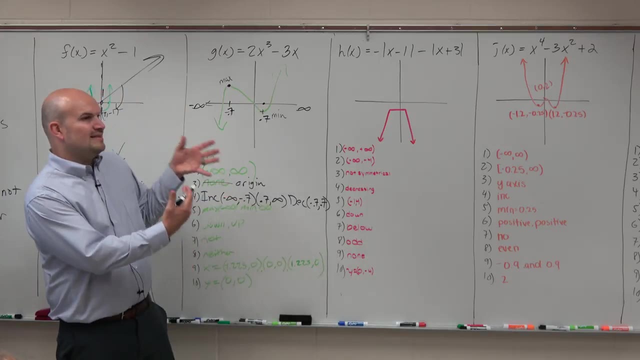 Watch what happens as I kind of like zoom in here Is now at a minimum. Yeah, It kind of looks like an absolute minimum too, right? So we know, based on the end behavior of this, that this graph is never, that's never, going to be the minimum, because we know the. 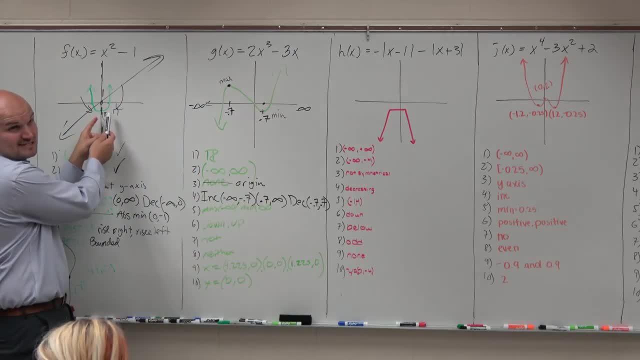 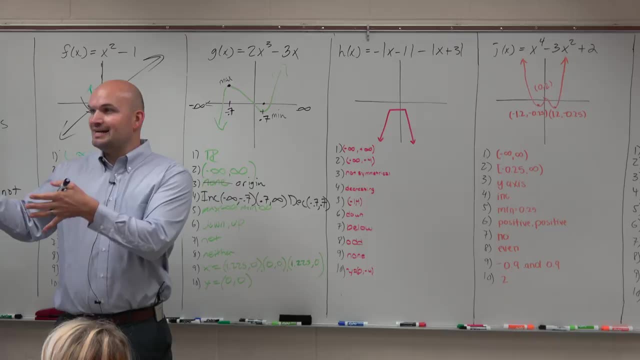 graph continues going down right, And there's no reason for us to believe, at least looking at this graph, that it's going to shoot back down right. We can just assume it's going to continue that way. So what's happened is what I just did, is I like zoomed in, I got more close, right, So you? 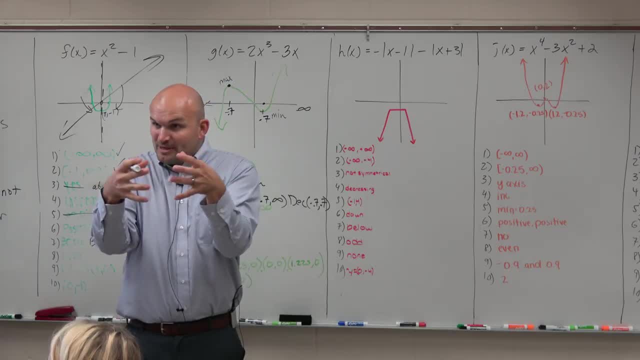 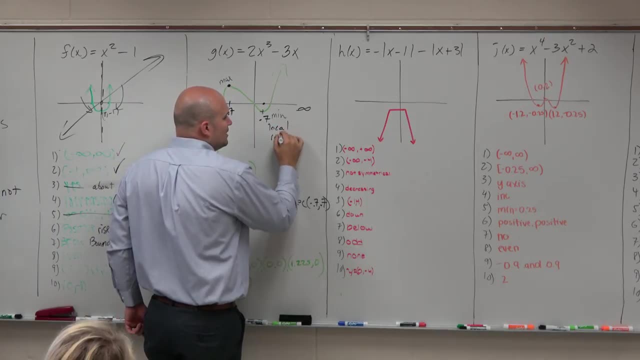 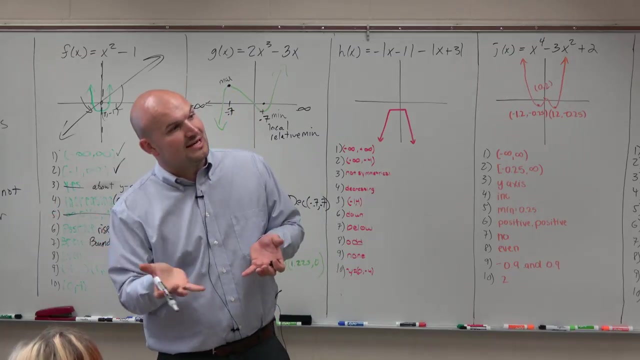 can kind of think of, like your relatives are the close people around you, The local people are like closely around. So we call this. it is a minimum, but it's a local min or a relative min. It's not the absolute min. The absolute min would be the absolute lowest that the graph goes. But when? 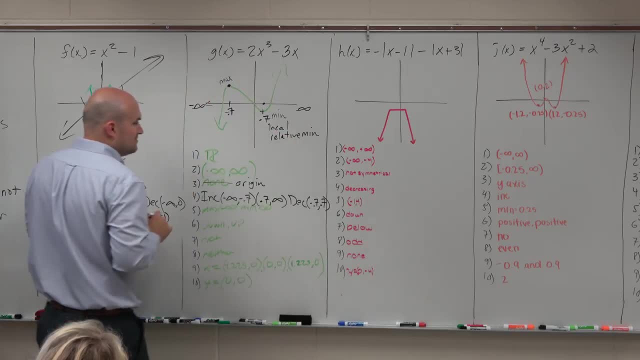 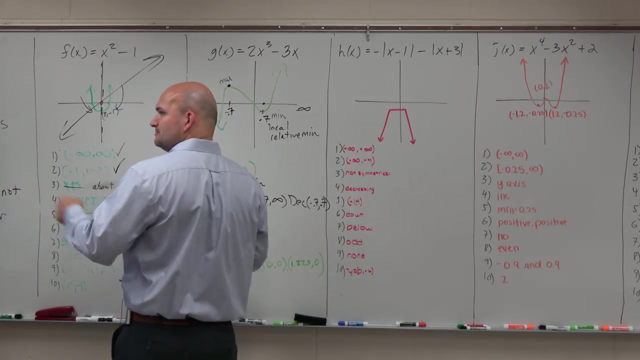 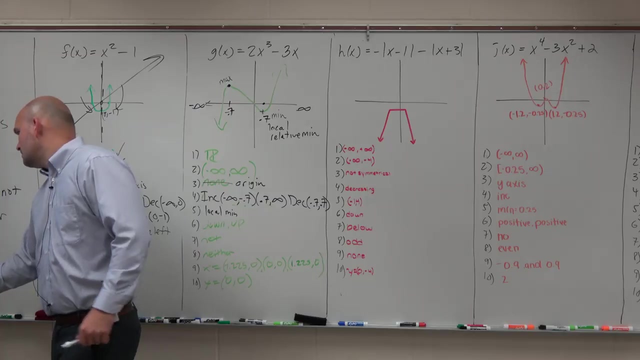 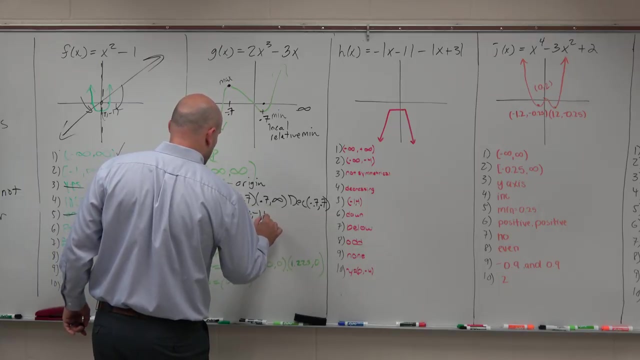 you're not talking when I'm talking, then you'll know that this is the local or the relative min. We just got to plot those points which they just said. I don't know where the affinity came from. So the local min is going to be at negative point or 0.7 comma, negative 1.4.. And the local max. 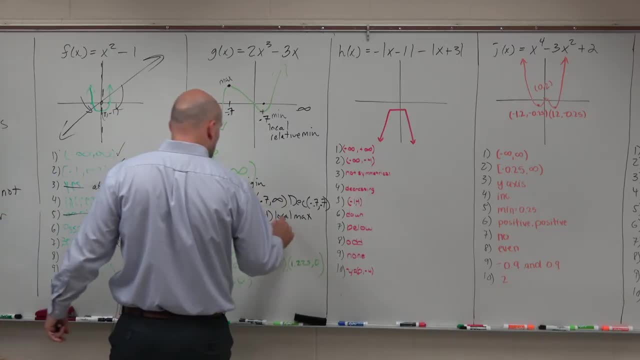 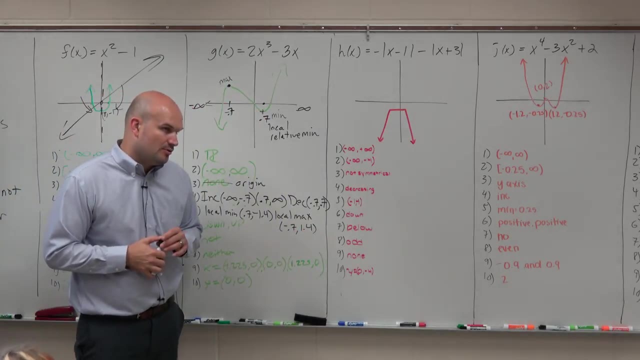 again. guys, I asked for points, So you should have. you'd want to make sure you provided points. The local max is at negative 1.7 and 1.4.. Next thing is let's talk about end behavior. So again. 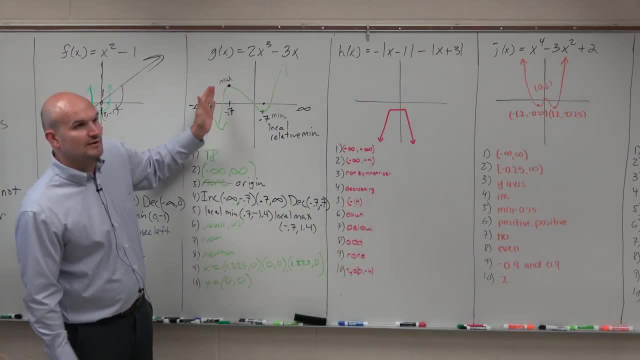 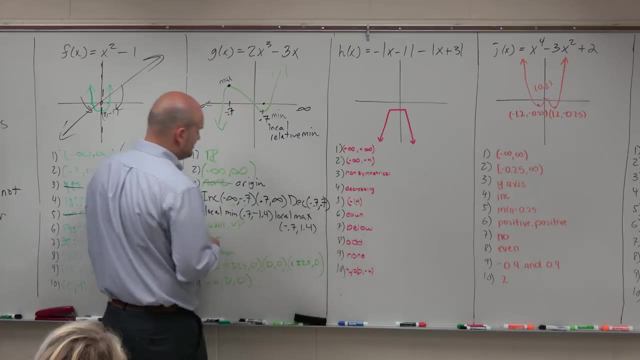 we can see that this end behavior, this graph, is continuously going down, And then, as we move to the right, the graph is going up. So what we can say is: down, up is, I mean, probably acceptable. I would just like to say: falls left, rises right Again. for right now I'm going to 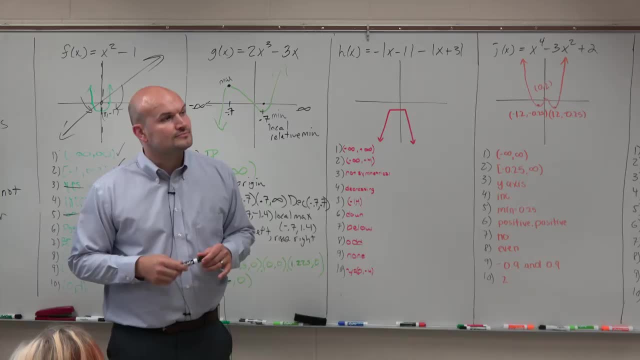 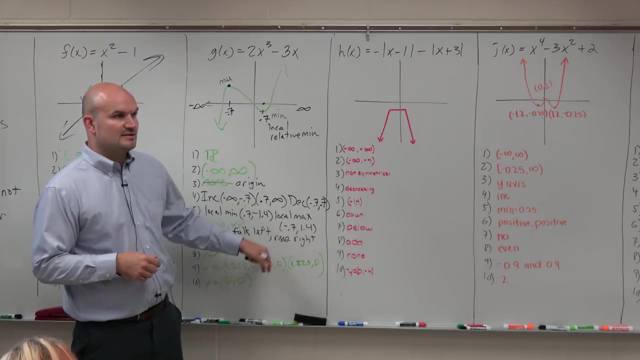 say that's acceptable, but we will get talk more about end behavior in a second. Yes, What term do you prefer? As in rising and falling? Yeah, I would just prefer rising and falling. To tell you the truth, we're not. this is just. 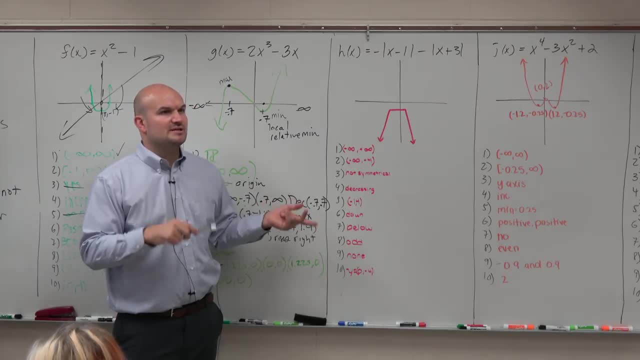 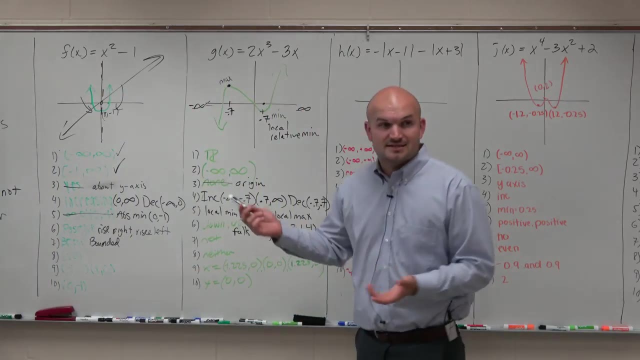 review stuff. I'm going to give you the way I want: end behavior, but that's not going to be until next chapter. Okay, So for I mean this whole activity, it's fine. The next one, number seven, is bounded Guys. does this graph have any boundaries going down low or? 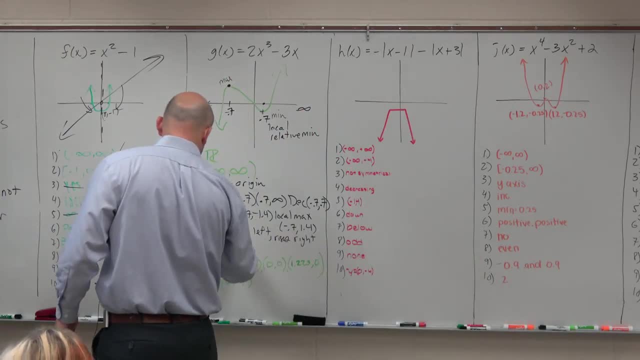 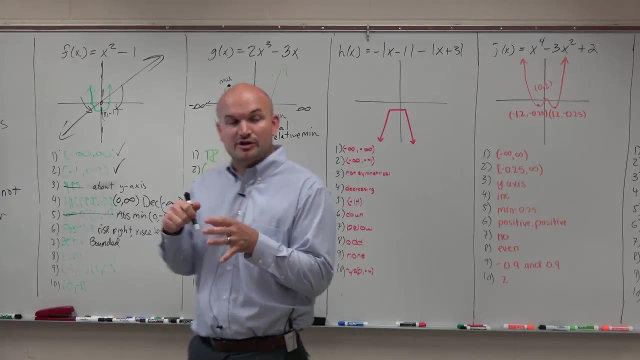 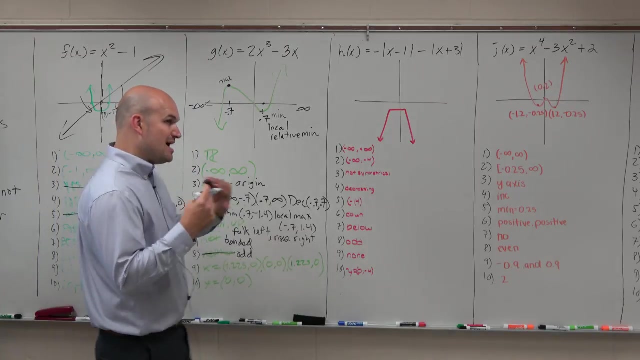 going up high? No, So let's say it's not bounded. Number eight: is this graph even odd or neither? So, based on the symmetry, whenever the graph is reflexive about the origin, it is actually odd. So when the graph is symmetrical about the y-axis, it's even. When the graph is. 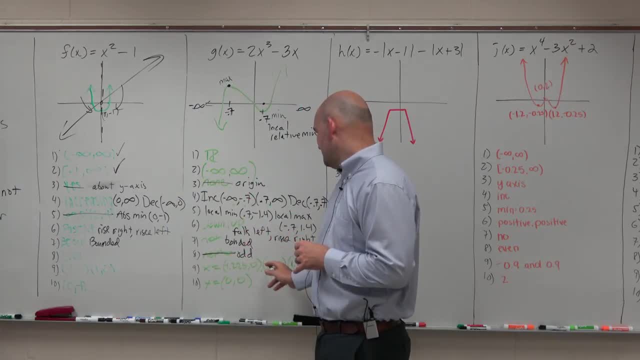 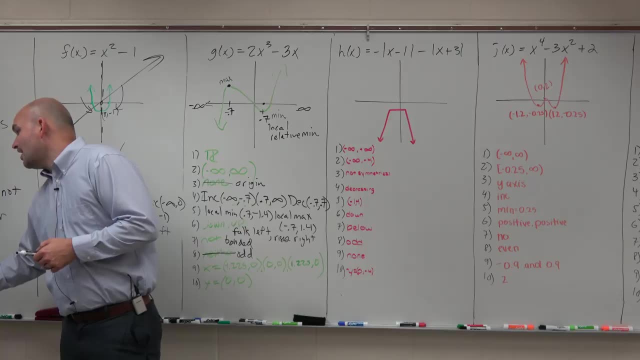 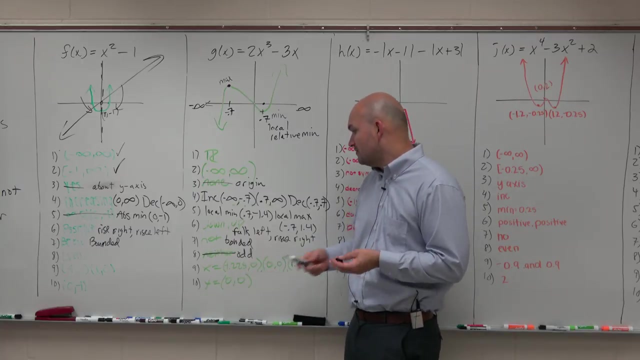 symmetrical about the origin. it's odd. All right, So I'm going to go ahead and get rid of all the points of the x-intercept which look good. I'm assuming Again, all I asked guys were for the x-values, I didn't ask for the points. 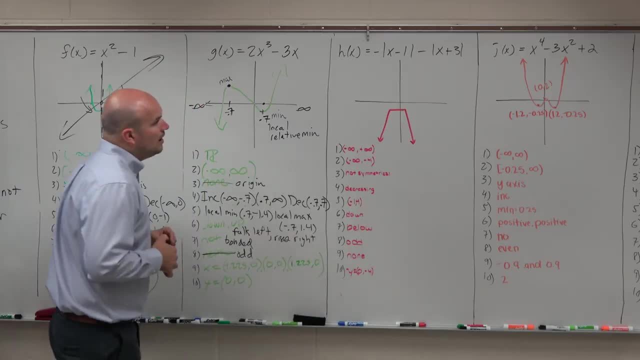 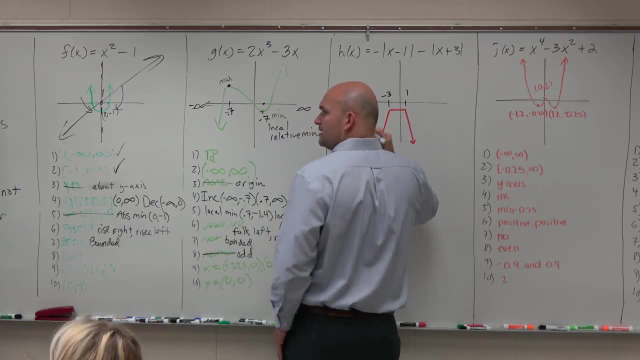 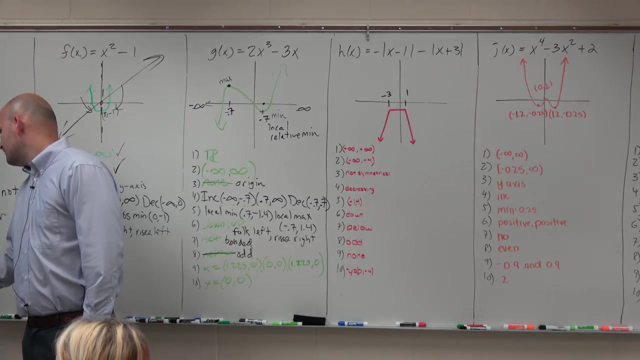 So you could have just done the x-values, because all the y-values, we know are zero. But that's perfectly fine from there, All right. So moving on to the next one. What's that a negative one? No, it's negative four. Oh wait, Did I type it in right? 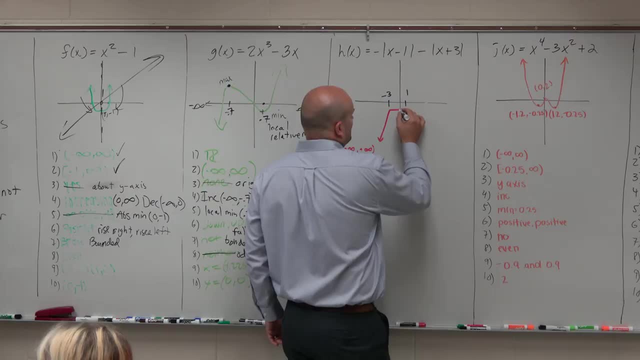 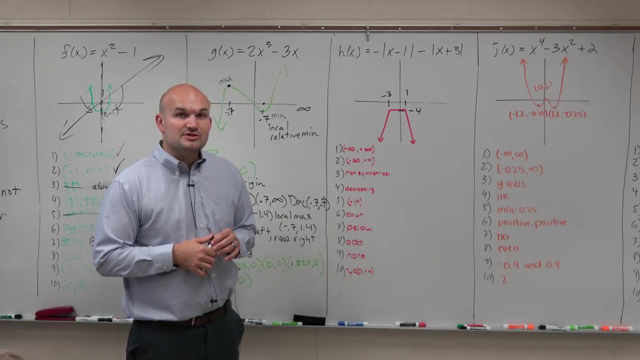 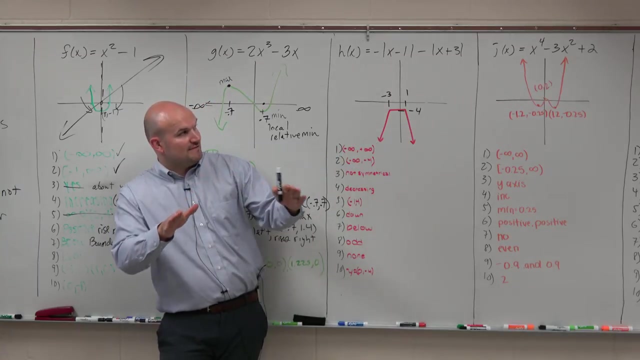 Yeah, Yeah, OK, So let's go and look at the next one. So the next one: we're looking at the domain Again. guys, it looks like this graph is going to continue expanding from the left and from the right right Indefinitely, So the domain is negative. infinity to infinity. Good job. 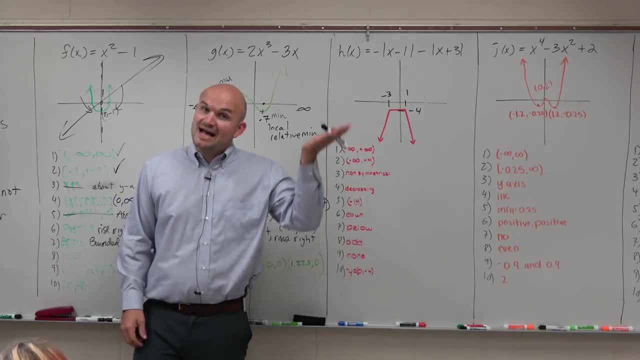 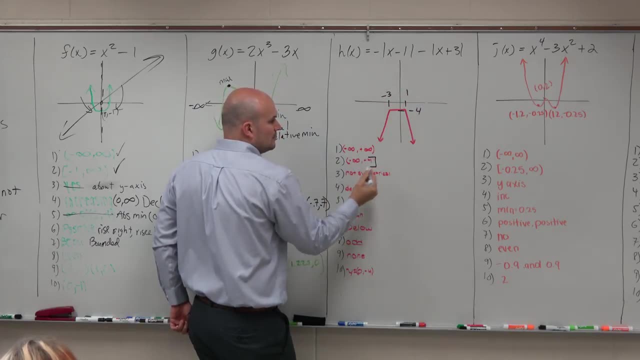 Yeah, So the change is basically from the graph. How low does the graph go to? how high does the graph go? You guys can see that this graph is going all the way up to negative four. Negative four is included, though, So we want to make sure we use the brackets, not the parentheses. The next thing: 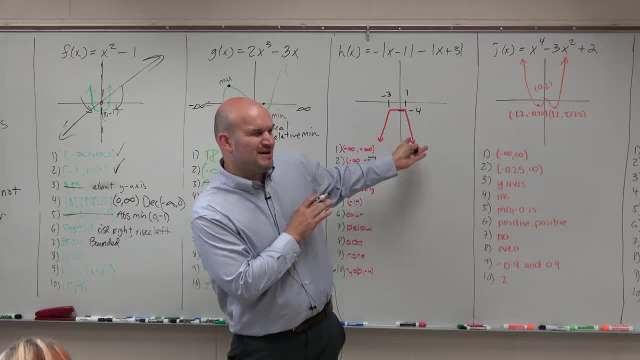 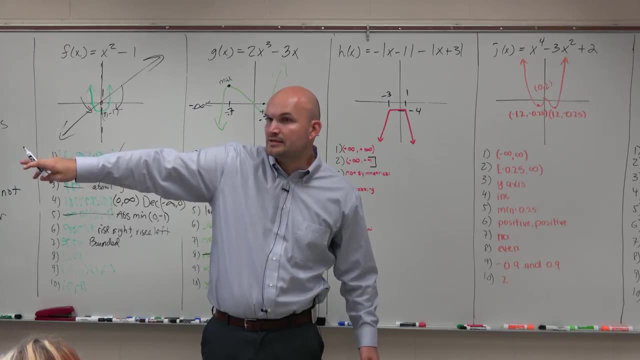 is not symmetrical. You guys might not be able to see it from there, It might not be perfectly clear, But obviously if you guys look at there, it is not reflective about the x, the y or the origin, right, That's pretty obvious looking at that. So that is correct. The next one is: 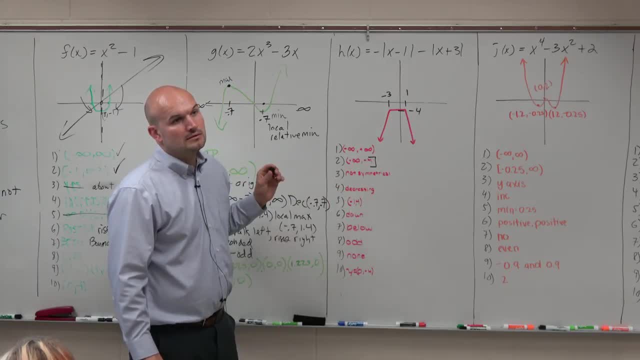 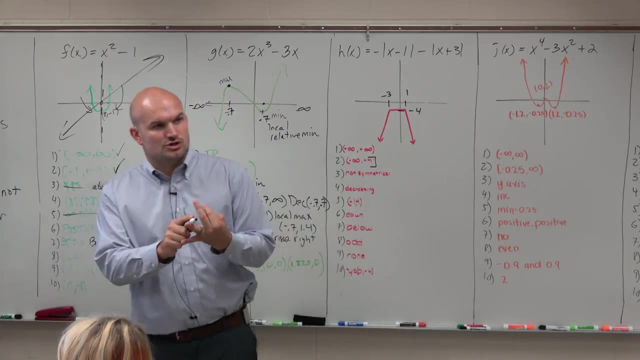 decreasing. Yes, Is it symmetrical around a certain point or like one? We're only going to be talking about symmetry from the x-axis, y-axis or origin. OK, Because yeah, you could say it's symmetrical about what Y equals like negative one if 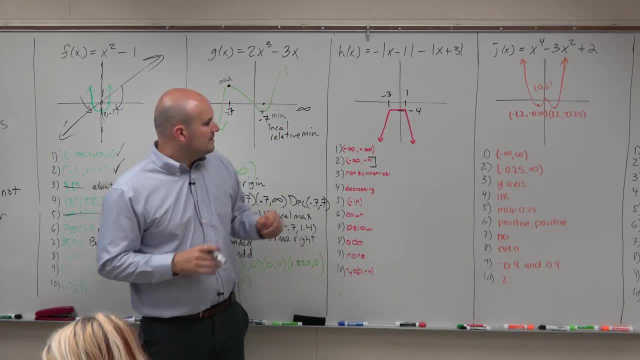 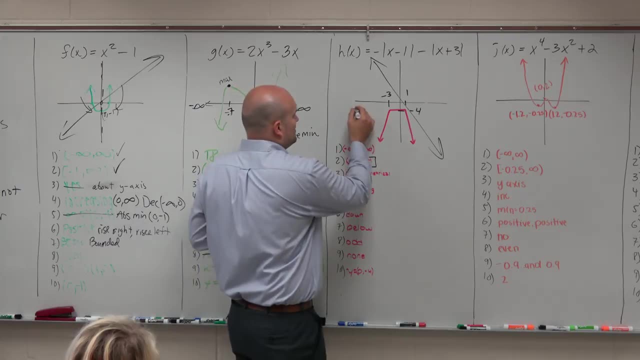 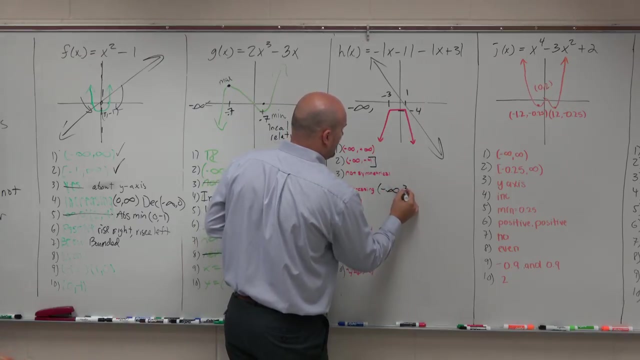 you wanted to, or Yeah Yeah? The next one is decreasing. Guys, this graph is not decreasing. Decreasing graph looks like this: right And plus. what about from negative infinity to three? On that interval from negative infinity to three, what is the graph doing? From negative infinity to three? 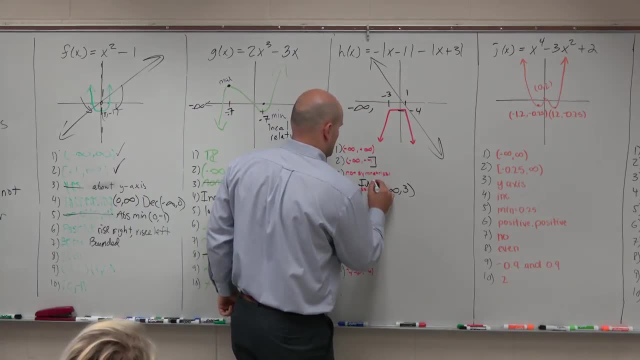 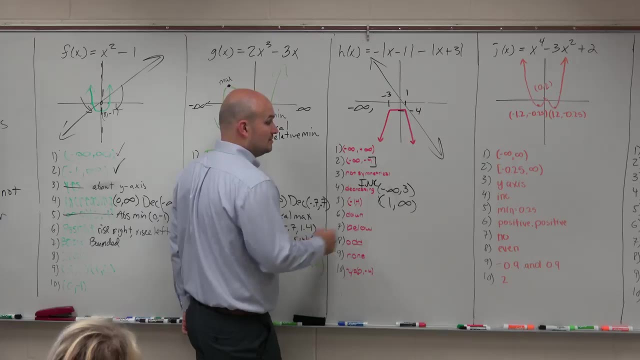 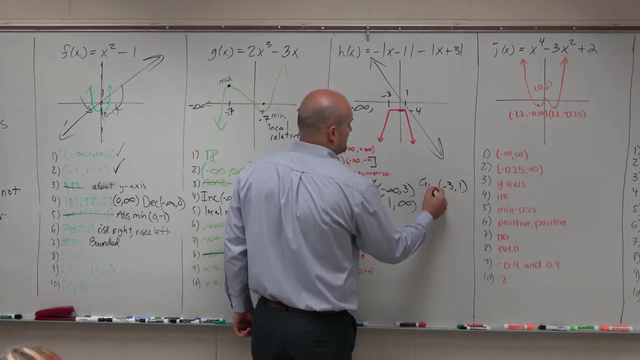 what is that graph doing Increasing, Increasing, From one to infinity? what is that graph doing Decreasing, Decreasing? And what about from negative three to one? It's constant, It's constant. OK, Just remember, guys, we write our intervals using the x values, OK. 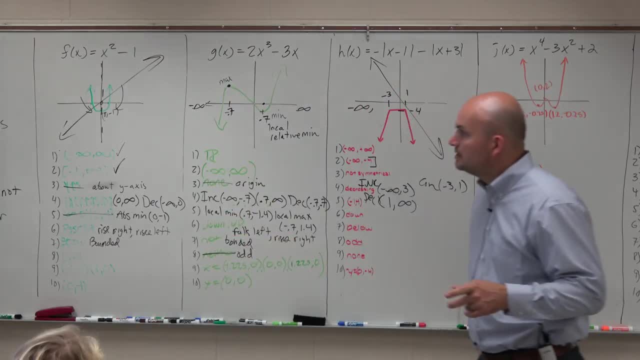 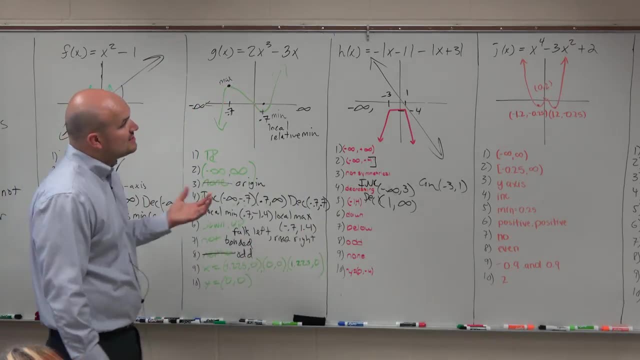 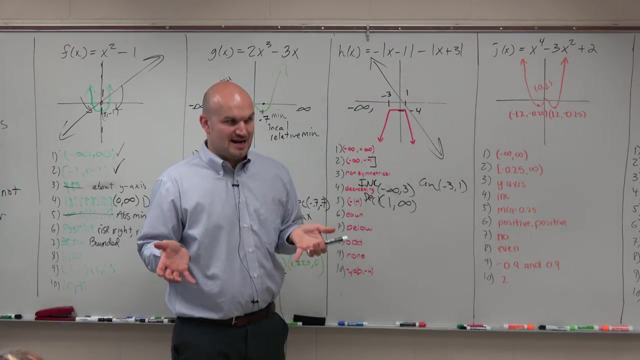 Next one is the maximum intervals, number five. So the- oh wait, max. yeah, the maximum points, not intervals, maximum points. So this one has, like this, max value at negative four, but there's not an actual point that makes up that value. There's not actually. 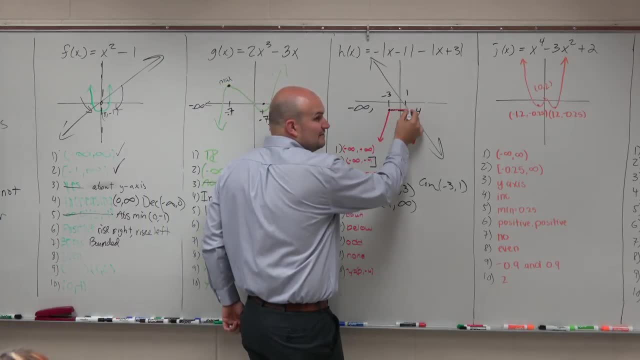 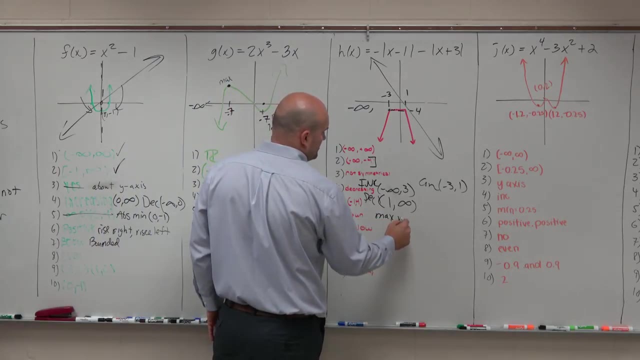 a point, because there's like constant values, That's an infinite set of points. So we can't really say there's a maximum point in this case. but we could say there's a maximum value of the graph And that maximum value would be: y equals negative four. OK, So there's really not a point. So 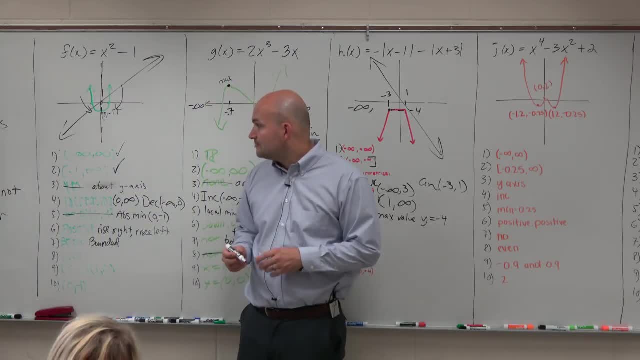 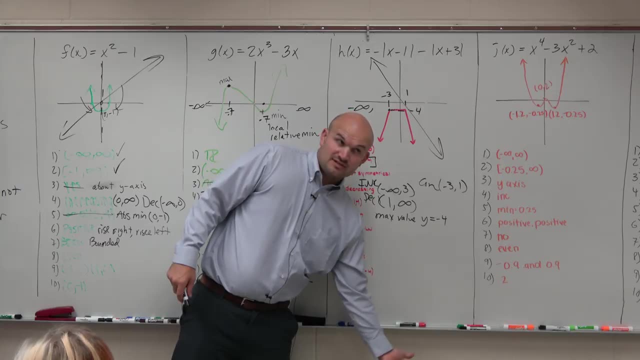 there's no point you could give. but you could say: there's a maximum value of the graph. Is the graph bounded above, below or not bounded at all? So again, guys, you can see the graph continues going down indefinitely. so it's not bounded below, But as it's continued, 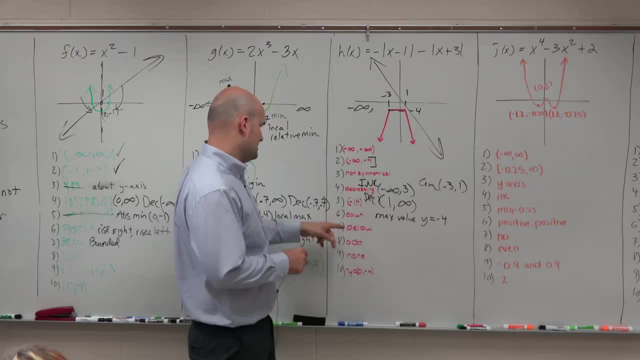 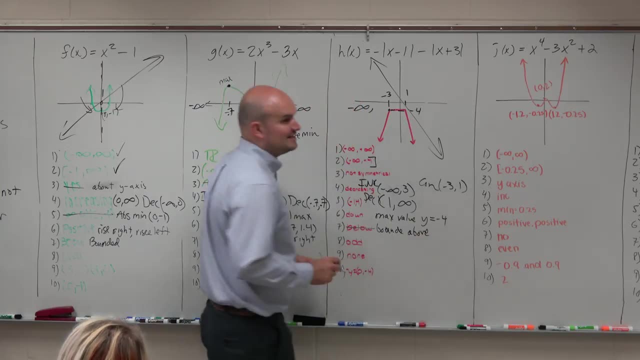 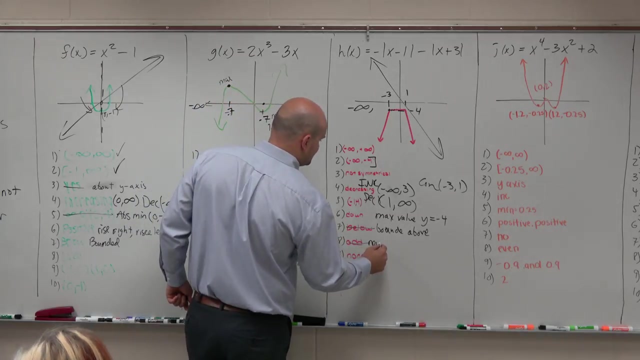 going up, you can see it is bounded above. So it is bounded above Since there is not any symmetry. remember guys, y-axis is equal to negative four, So it's not even Origin is odd, Since it has no symmetry. it is neither, It never crosses. 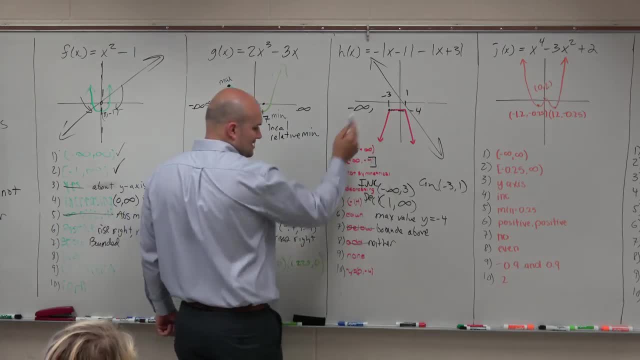 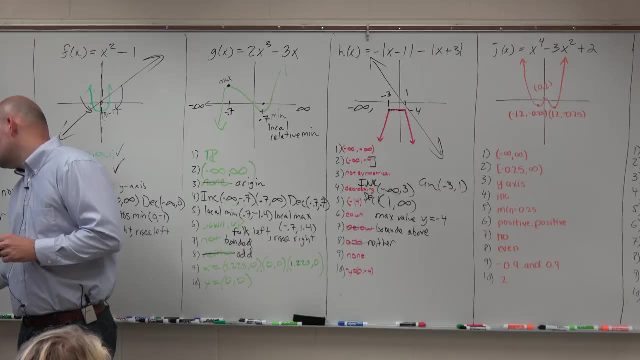 the x-axis And then the y-axis crosses at zero comma negative four. Good job, Moving on to the last one. All right, On to the last one, guys, and then we'll be all done. So this last one, they graphed. it Looks like the domain is from negative infinity to infinity. Good job. 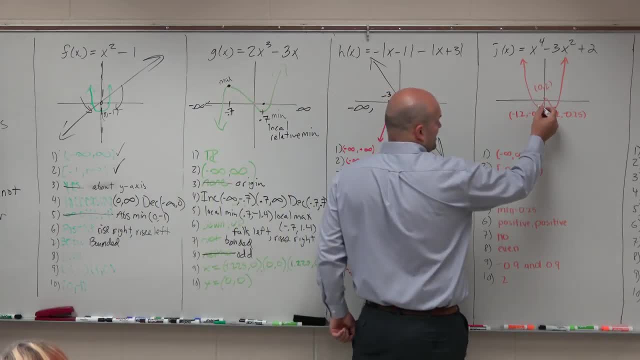 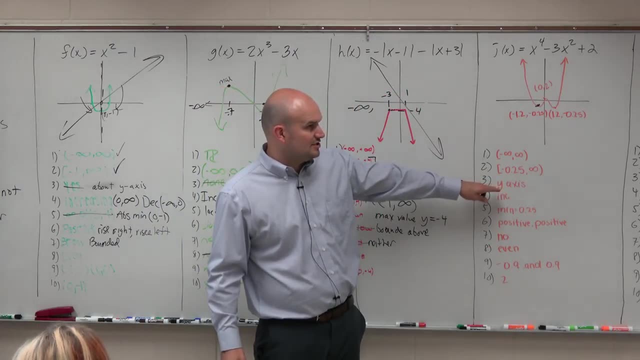 The range is from negative 0.25.. That's what that point is. Very good. Negative 0.25 to infinity. Good job, The symmetry is about the y-axis. Good job, The symmetry about the y-axis is good. 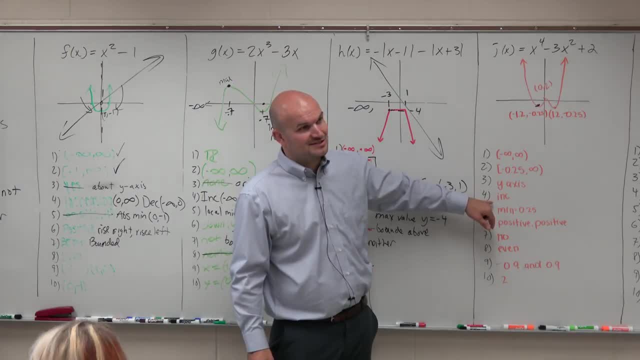 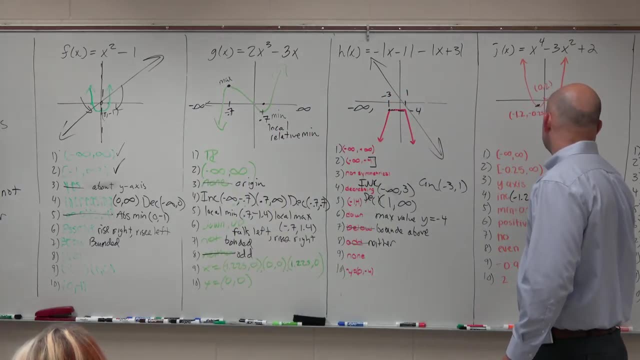 The graph is not increasing. Now you guys can see this is increasing, But where is it increasing? It's only increasing on an interval of negative 1.2 to 0.. And then it's increasing on the interval 1.2 to infinity. Right, You guys agree, Here is increasing, Here is it. 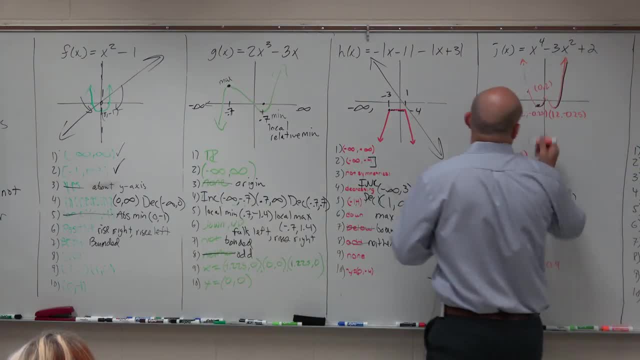 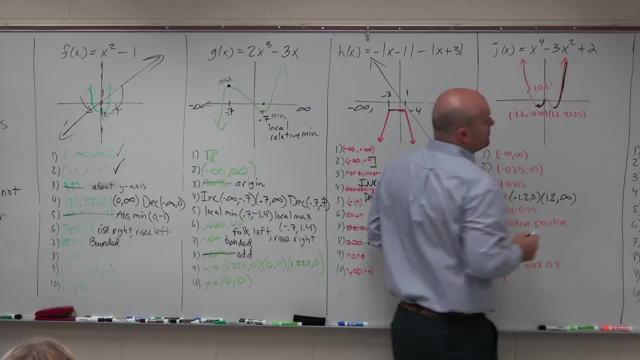 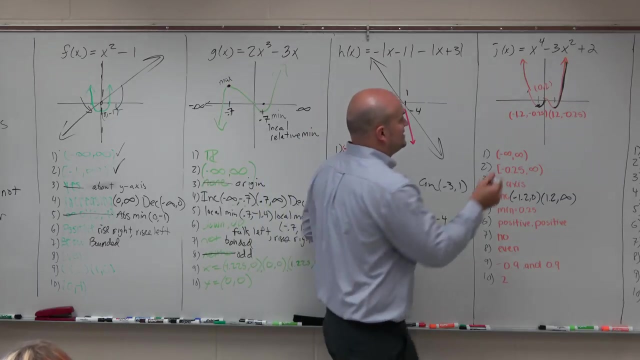 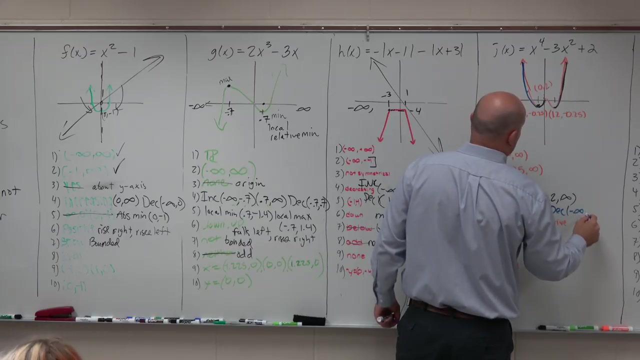 increasing. Go back to your orange Right. You guys see the black Of it increasing Right. So you're only talking about the x values. where it's increasing, Then it's decreasing, But it's only decreasing from negative infinity to negative 1.2.. And 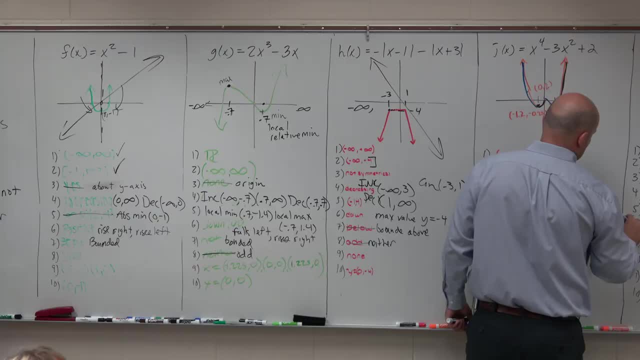 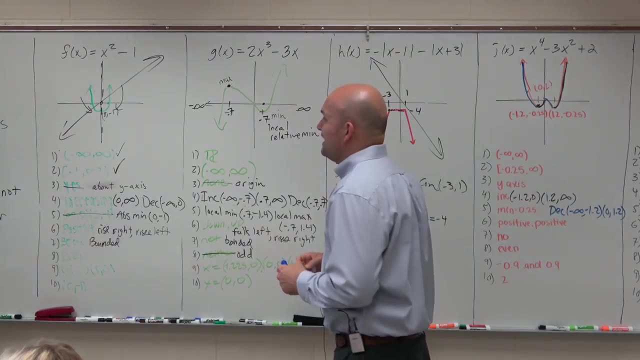 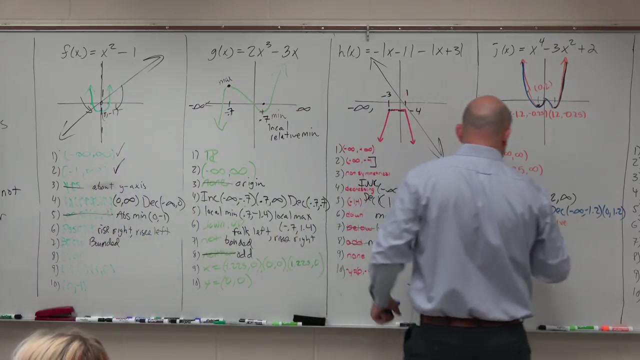 then it's decreasing from 0 to 1.2.. I hate to have to change seats already. Number six: M: behavior, Positive, positive. So, ladies and gentlemen, again you guys can look at this. The graph is rising from the left and from the right. So we just say: 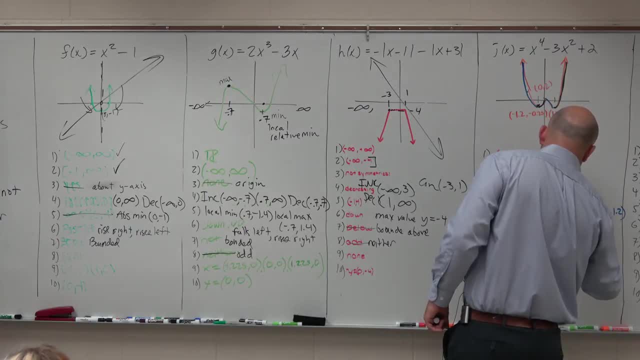 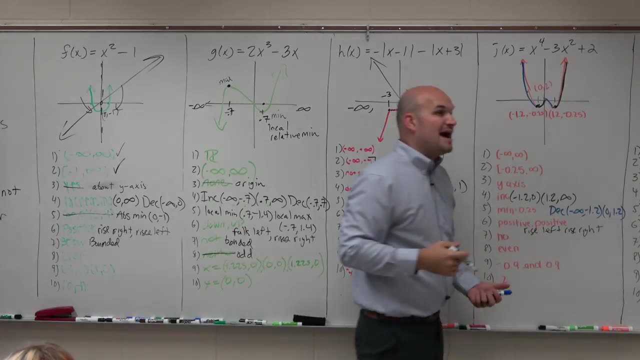 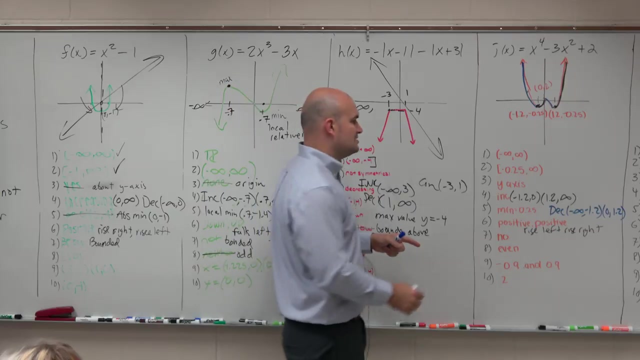 you know, rise left, rise right. Oh, I forgot to do number five, which is the max min points. You guys can see there's two minimum points and they're both absolute. It's okay to have more than one absolute minimum or more than one absolute maximum. So we're going to say: 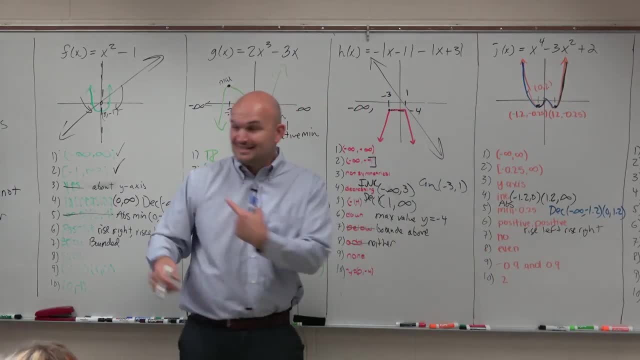 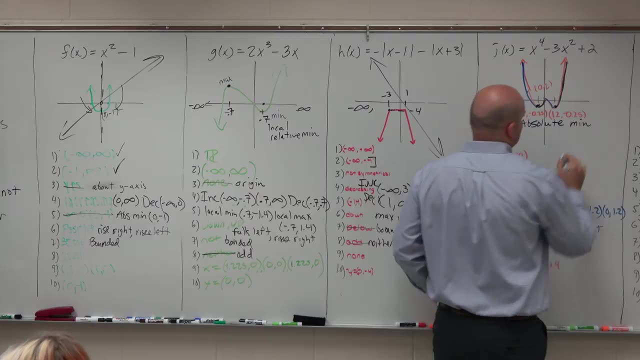 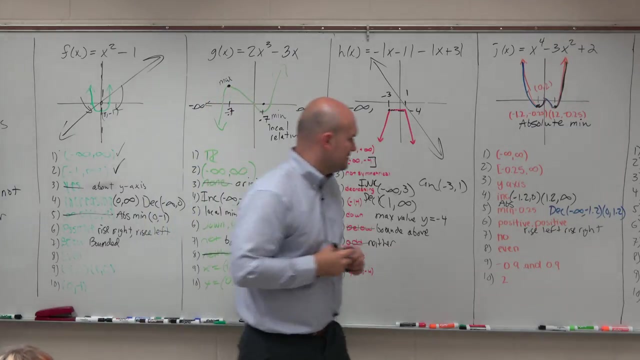 just make sure you label them as absolute Absolute minimum. And again, I did ask for points, So actually I'll just label them here: Absolute minimum points. All right? Next one is number seven. Is the graph bounded above or below? You guys can see that the graph is bounded below right. 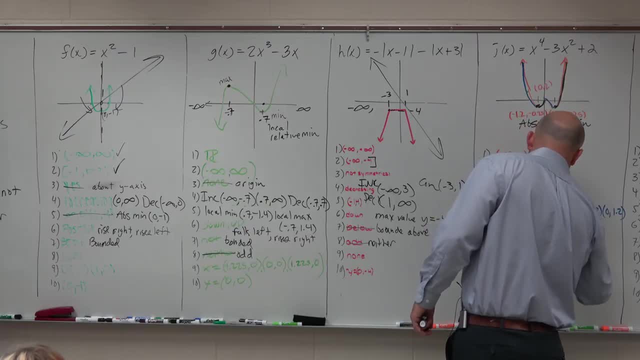 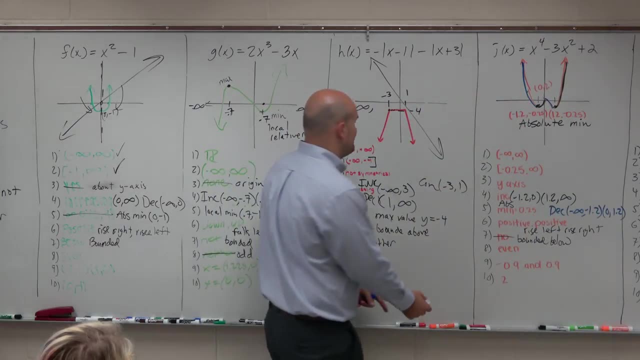 So it is bounded below. It is symmetrical about the y-axis, so it is even. And then make sure, guys, when you're doing these, just these values are not where the graph crosses the x-axis. I don't even know where point nine came from. 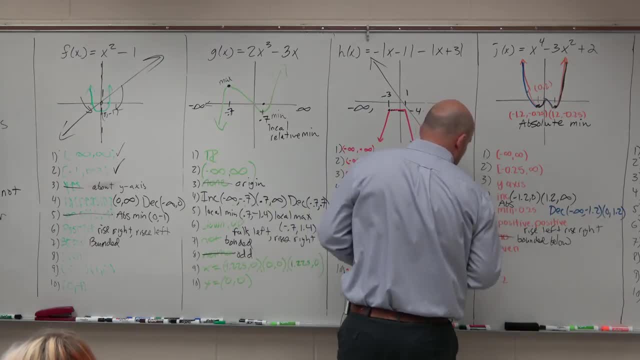 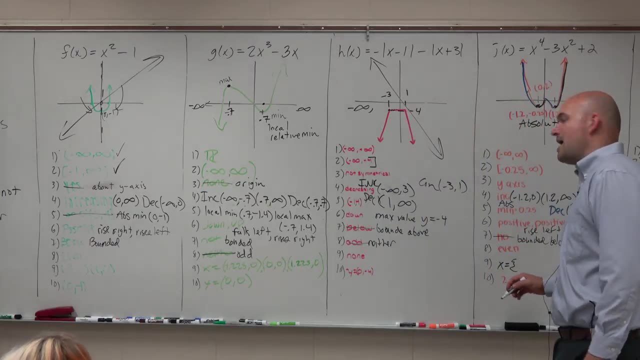 So you can go ahead and write them in there as values like x equals and then write them as a solution set Again. we're just looking for the y-values where it crosses the x-axis. So negative 1.4, negative 1, 1, and 1.4.. 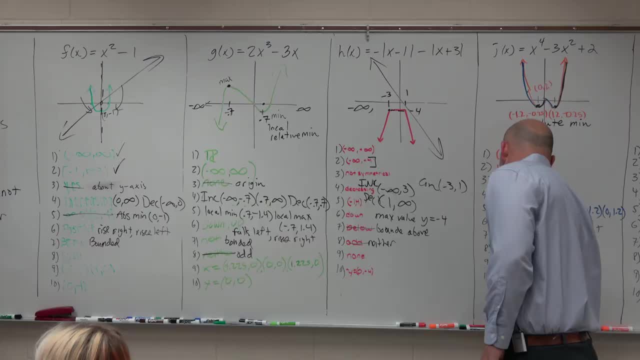 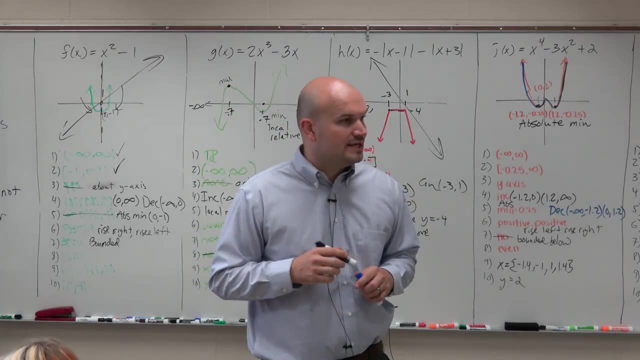 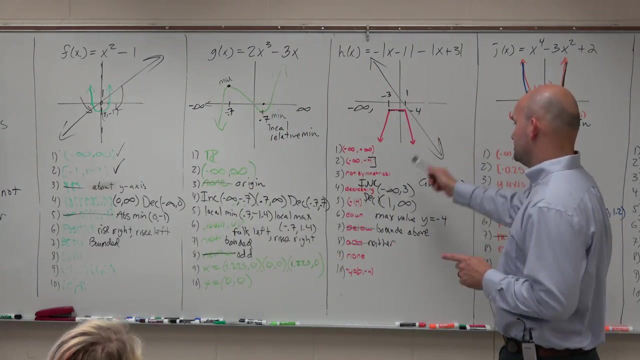 The y-intercept is going to be y equals positive 2.. Anybody have any questions on any of the graphs or the answers that I provided? Yes, You didn't do number six on the third graph. Number six on the third graph. 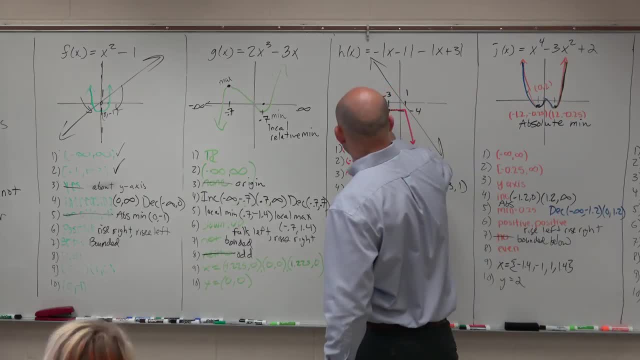 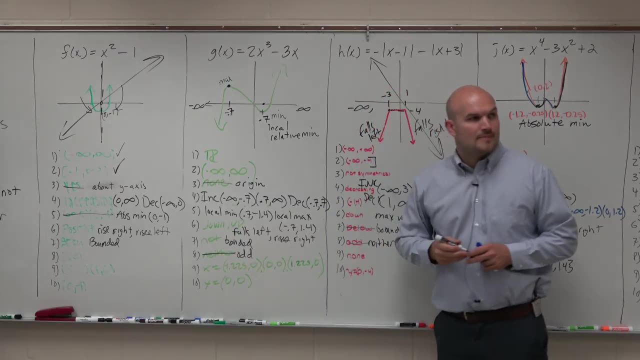 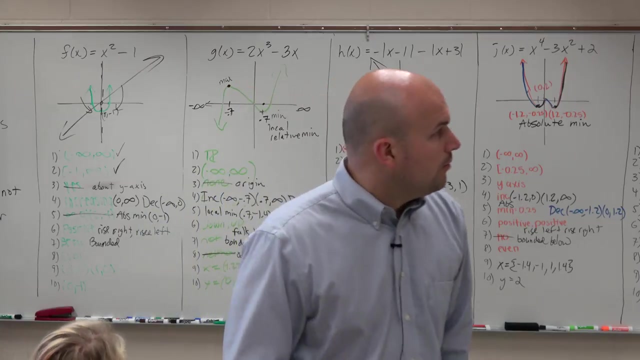 I didn't. It is falls left and falls right. Thank you, Any other questions, Any other ones I skipped, or anybody have any questions? Okay, Well, ladies and gentlemen, make sure that you guys have your answers to.